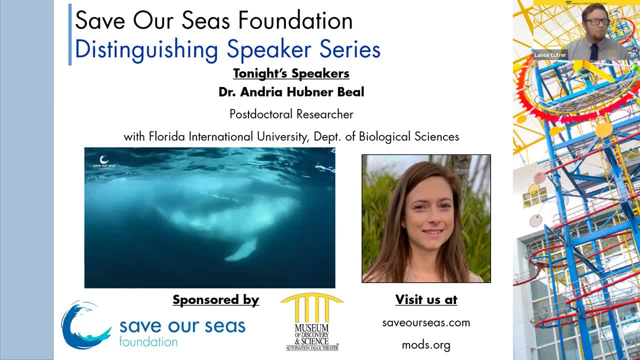 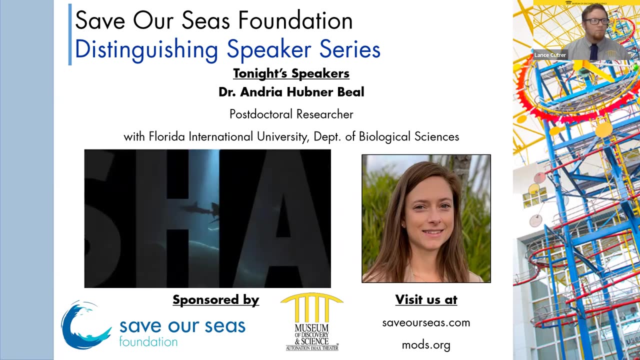 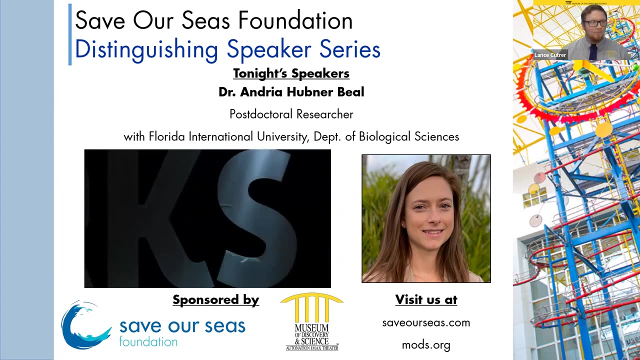 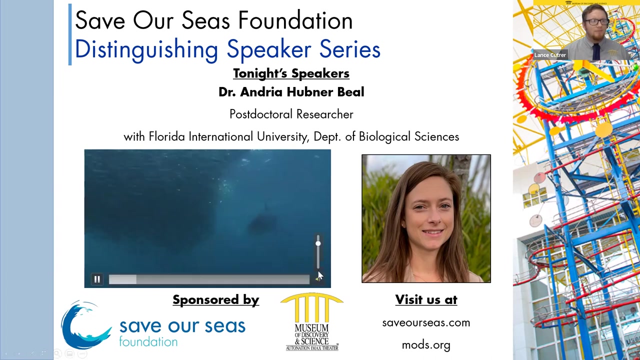 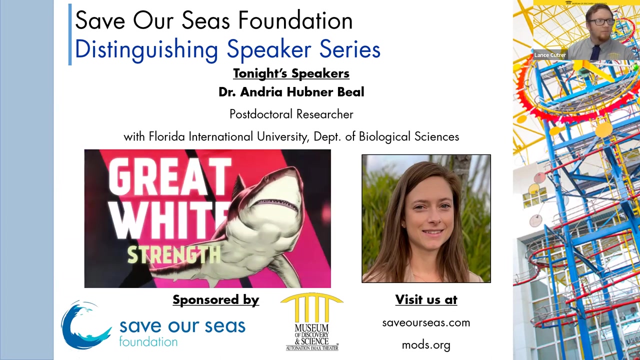 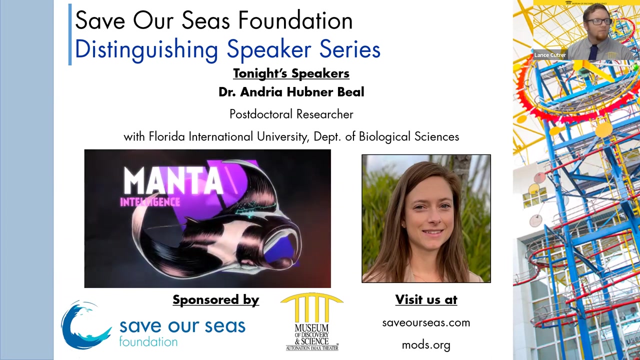 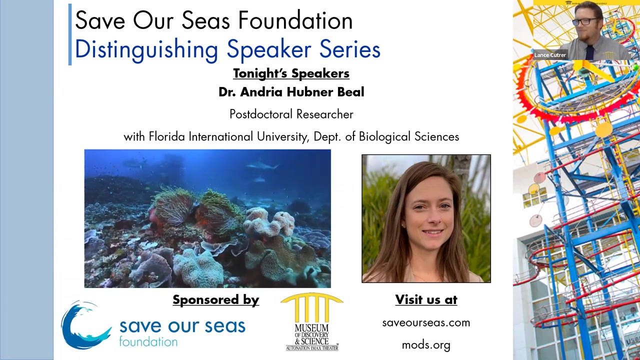 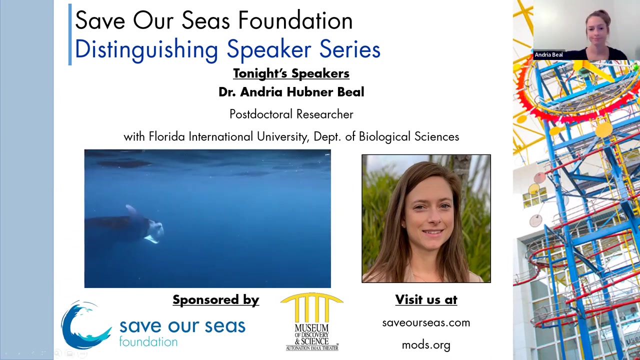 We can and will make a difference. The Save Our Seas Foundation. The legends of the deep, Ancient and elusive. They are the keepers of balance in our oceans. Mountain chiefs were born big and strong. The current They are Sup Joshua. Together they ensure the stability of our world's life, support the oceans. 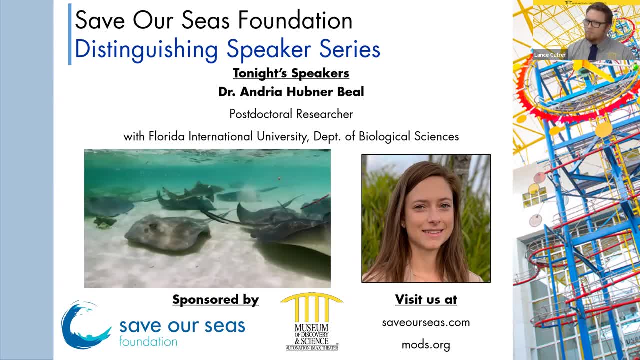 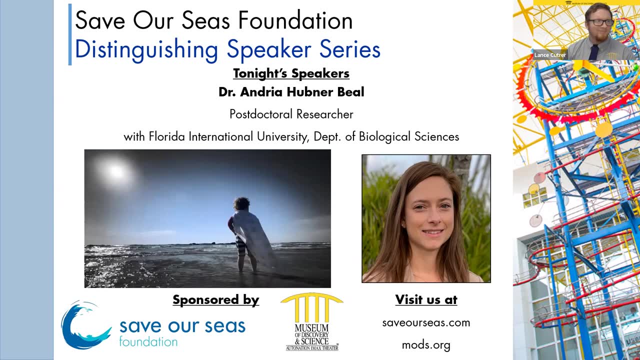 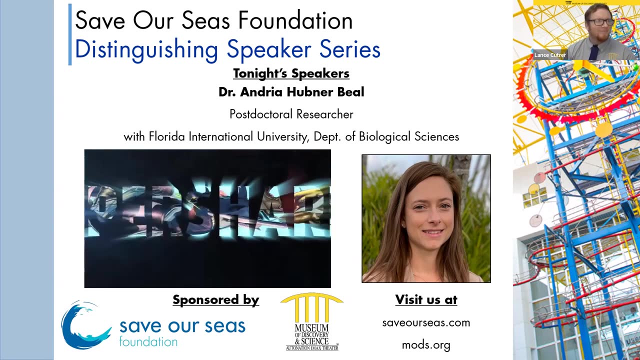 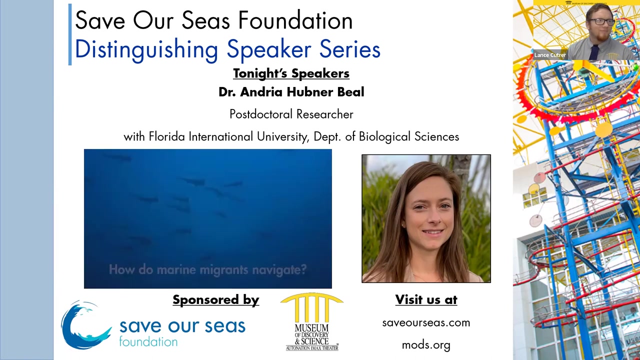 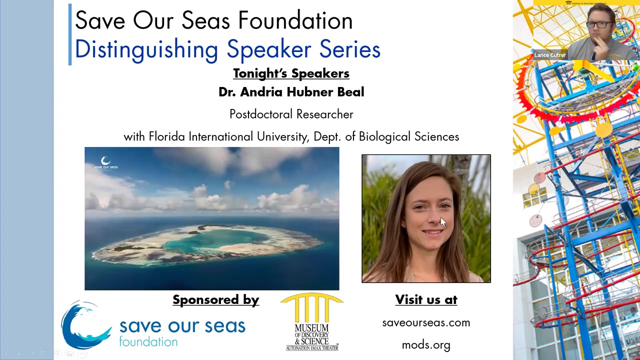 Our oceans need super sharks. we need them and they need our help. Assemble the super sharks and help them save our seas. Sharks and rays. we are ancient, eclectic, misunderstood and essential to our oceans, But these important animals are the only means of life support. 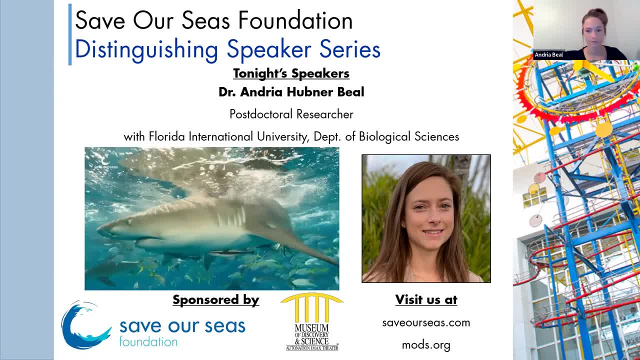 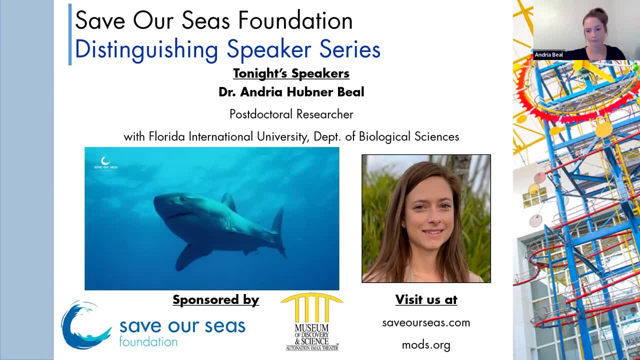 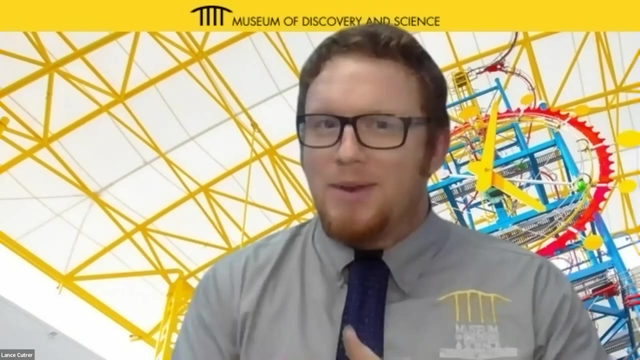 As the Save Our Seas Foundation. we are here today for supporting research, conservation and education. We work to ensure people are safe. We work with sharks and rays to save our seas foundation. Together we can make a difference. All right, Well, welcome everyone to tonight's Save Our Seas Distinguished Speaker Series. 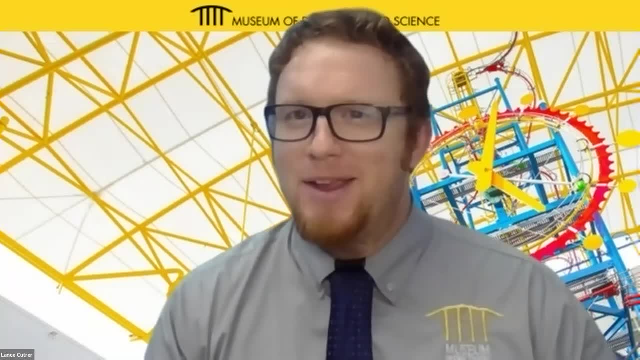 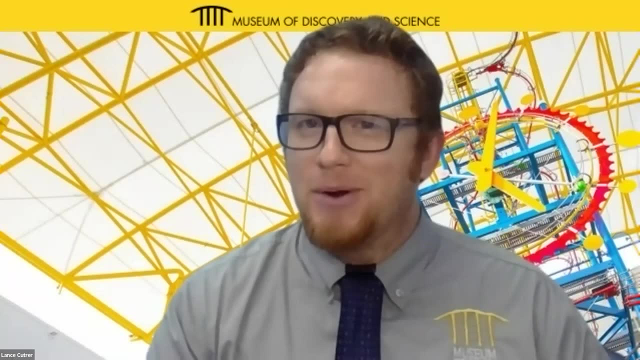 My name is Lance. I am the Director of Environmental Sustainability at the Museum of Discovery and Science. Tonight we're going to be talking about how to save our seas Tonight. we have a wonderful guest speaker here tonight to talk to us all about sharks and her research into lemon sharks in the Bahamas. 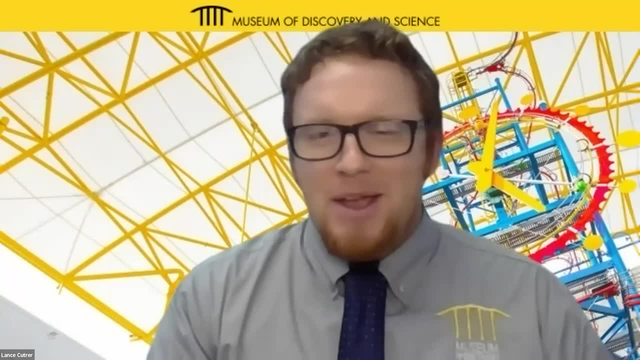 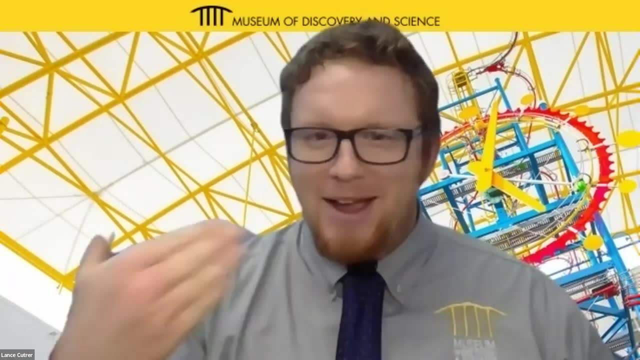 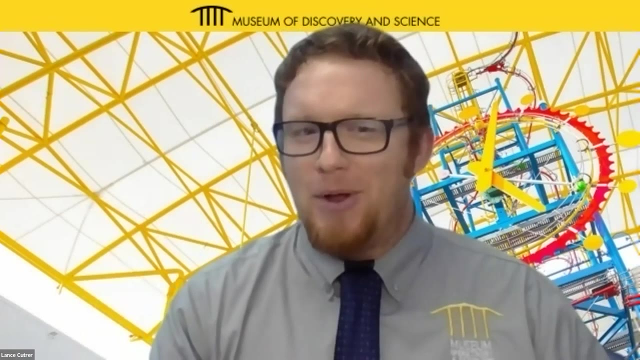 I'll introduce Dr Beale in one minute, But if this is your first time here, welcome For those of you that are repeating night after night coming for our Distinguished Speaker Series. thank you very much for joining us. We welcome all. 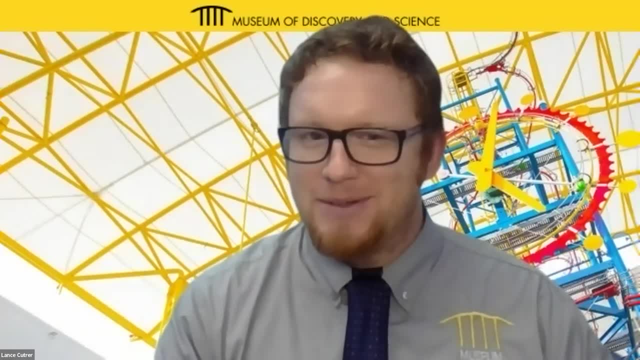 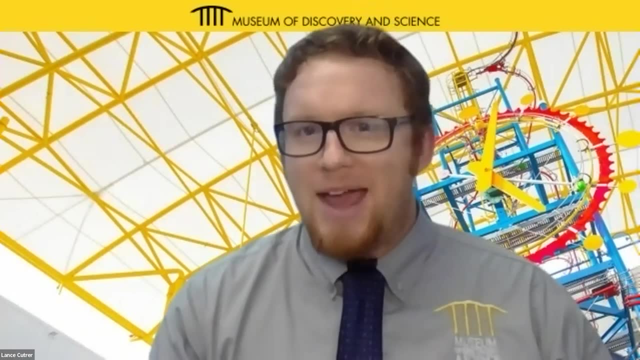 And we can't wait to see you again. If you have any questions for tonight, please feel free to ask questions as we go along. You can type questions in the chat. We ask that everyone just stays muted throughout, But if you have questions, feel free to ask. 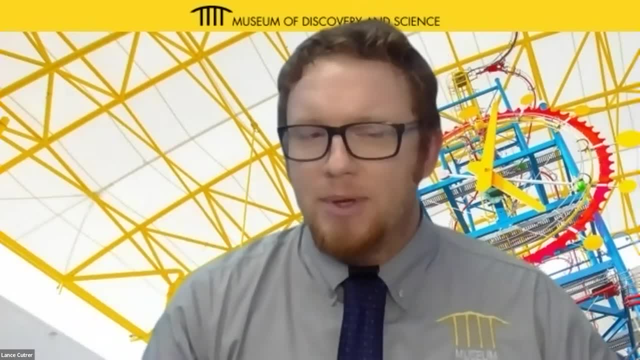 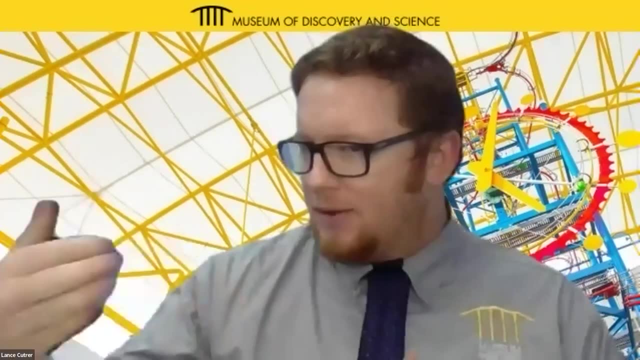 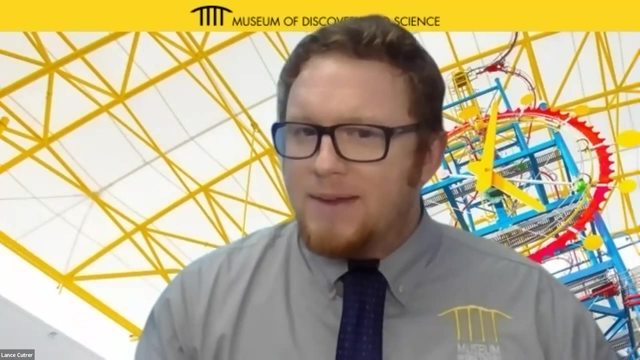 We'll be going in as Dr Beale is presenting to answer any questions you might have, So feel free, And towards the end of the presentation we'll have some time for question and answer as well. A few things about the museum. 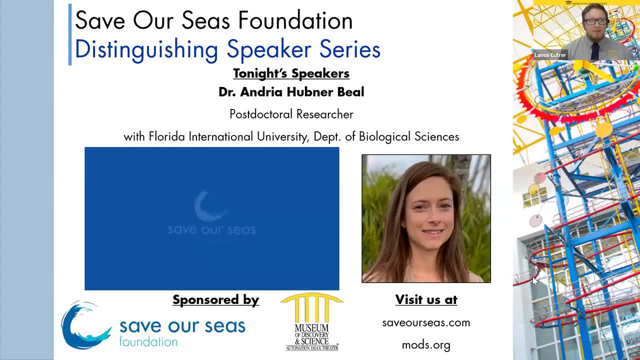 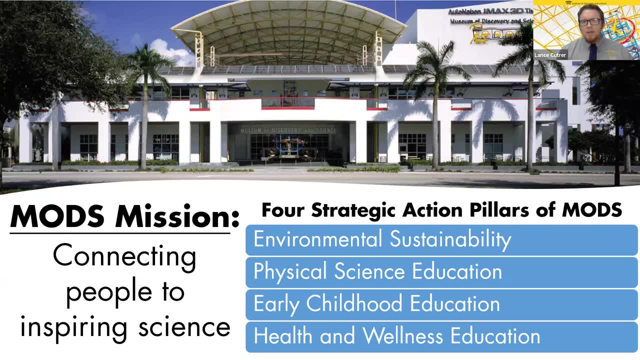 So we are the Museum of Discovery and Science. In the museum we're located in Fort Lauderdale, Florida. Our mission is to connect people to inspiring science. So to do that, We have four strategic action pillars that we highlight here in the museum. 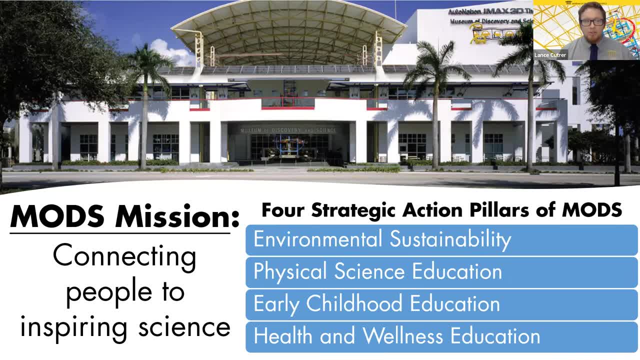 We highlight physical science education, early childhood education, health and wellness education and environmental sustainability. This is where the speaker series comes into play: to educate the public all about nature and the environment and have more stewardship for these places as well. The more you understand, the better. 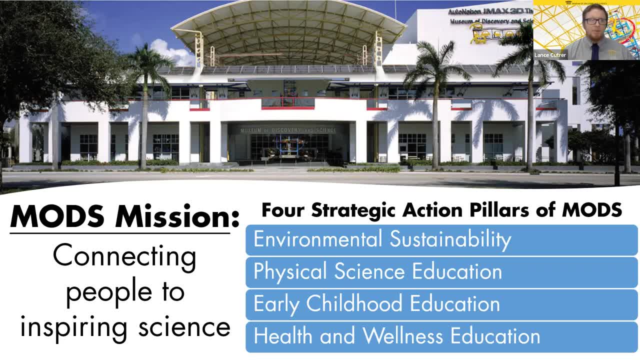 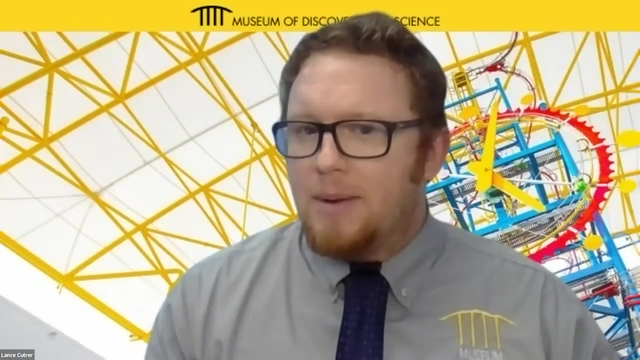 So that's a little bit about what we do here at the museum. Anyone is always welcome to come and join and explore. We have a lot to explore. We're for children of all ages, It doesn't matter how old you are. Tonight, like I said, we are joined by a researcher, Dr Andrea Beale. 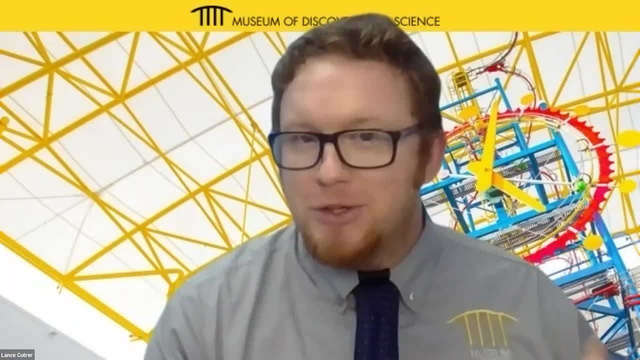 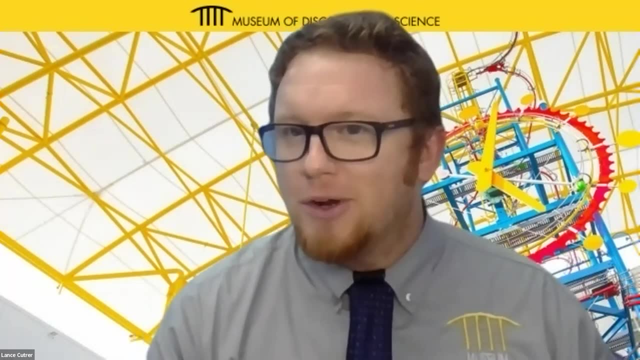 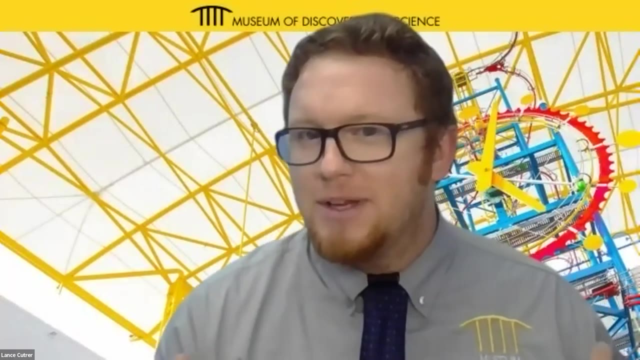 She is a scientist and entrepreneur. Her passion for sharks started in her youth, where family vacations to the beach and watching shark documentaries were among her favorite activities. Andrea's interest in conservation work and science has led her to currently study lemon sharks and the mohommans. 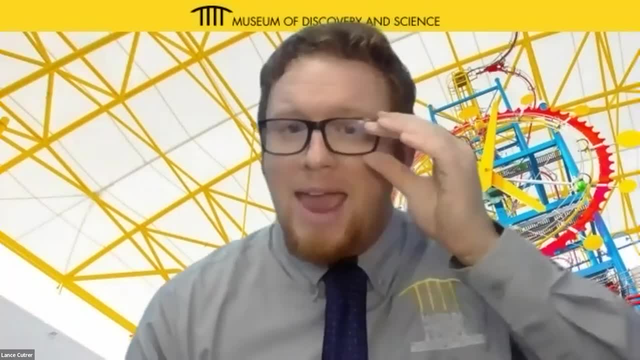 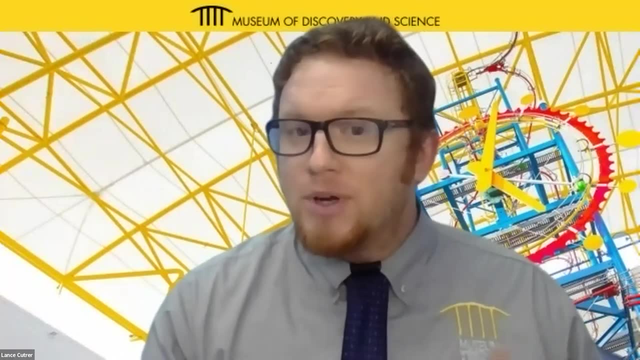 There she gathers genetic data from lemon sharks and analyzes that data to better understand the effects of pollution in the ecosystem. Andrea recently received a PhD in biochemistry. Andrea is a professor of biology at the University of Florida. She has a PhD in biotechnology. 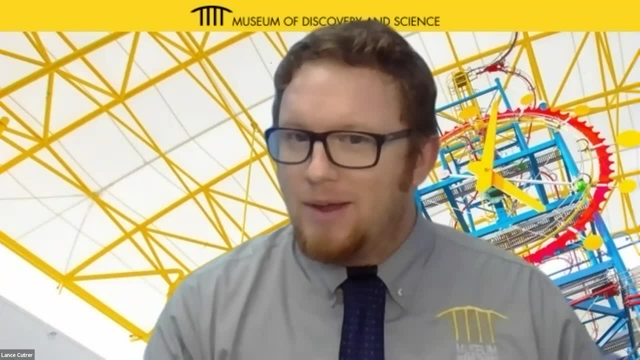 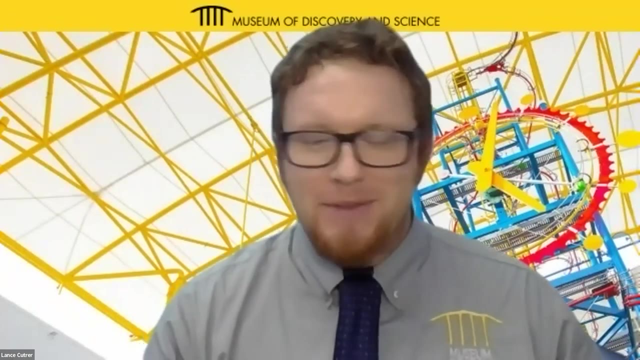 She is a professor of biology at the University of Florida. Andrea recently received her PhD from Florida International University in North Miami, Florida, in December, actually, of last year. So congratulations, Dr Beale. Andrea also currently runs a pet tech startup company called Epipaws, dealing with the genetics of pets. 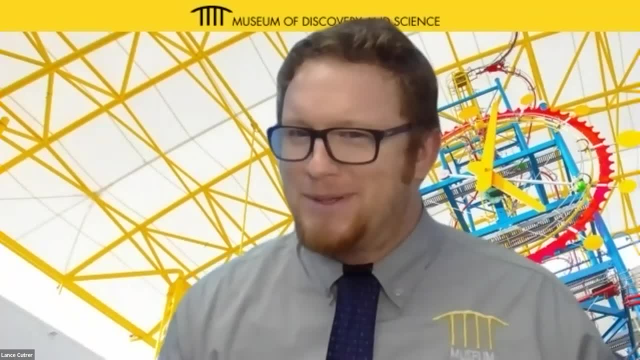 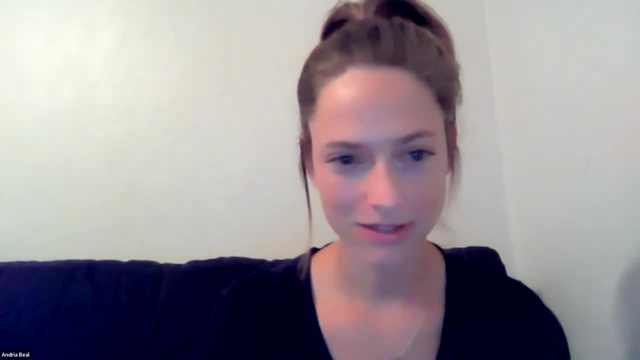 Interesting And owns a boat rental business in Fort Lauderdale, Florida. So scientist and entrepreneur, It fits quite well. Andrea is a scientist and entrepreneur. It fits quite well. It's a great description. Welcome, Andrea, Thank you. So let me share my screen. 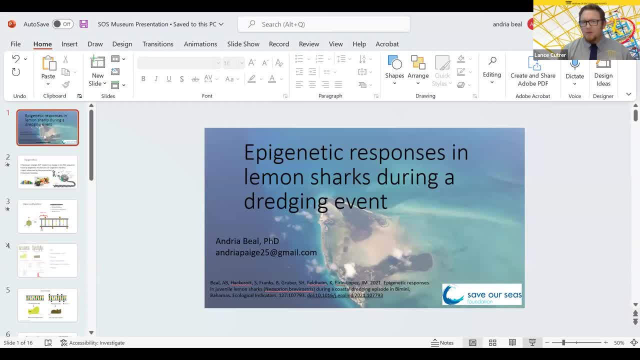 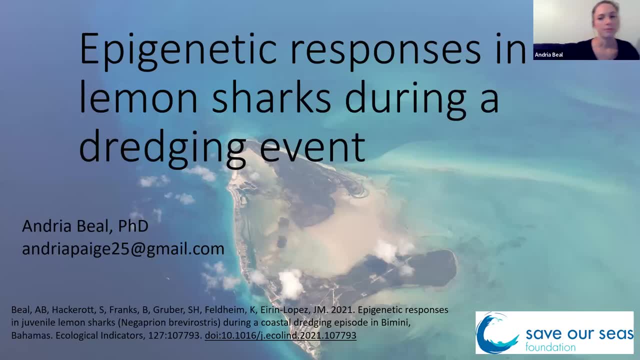 Yes, please do. And again, for anyone that has questions, feel free to type them into the chat. So, yeah, take it away. Yeah, please, And definitely while I'm speaking, if anyone has a question or wants to jump in, we can do that. 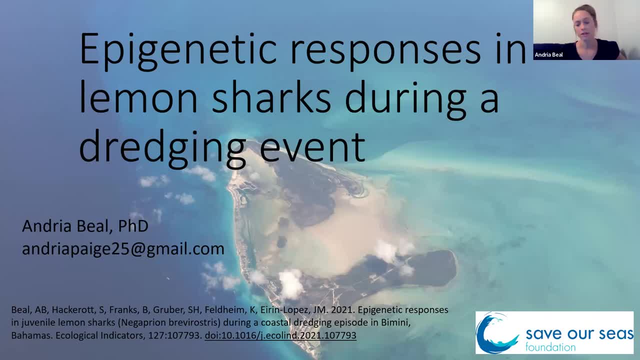 There you go or wants to jump in. we can keep this very conversational. I don't need to just talk all the way through this. If you have a question, just stop me and we can chat a little bit about what's going on, especially if you don't understand some things. There's a couple. 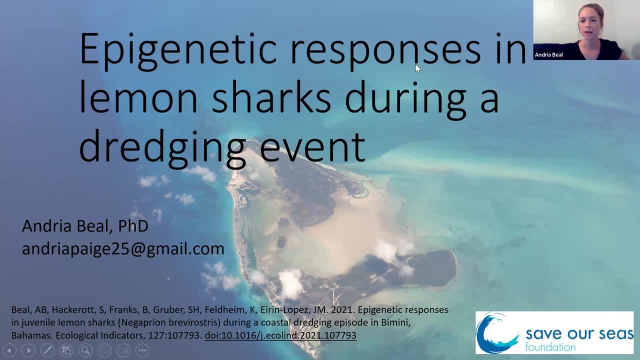 maybe new topics that I might explain, because what I looked at was actually epigenetic responses in these lemon sharks in response to a major dredging event that occurred in Bimini, Bahamas, and this was one of my dissertation projects that was funded by Save Our Seas and I did 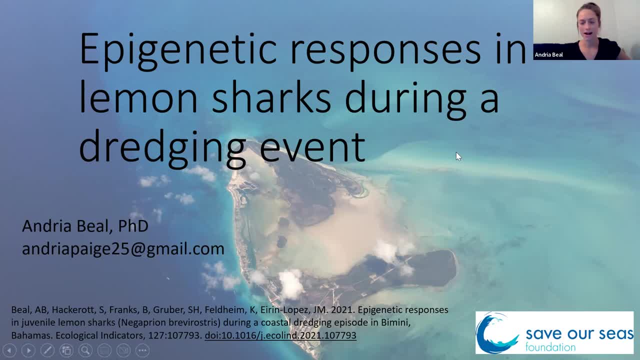 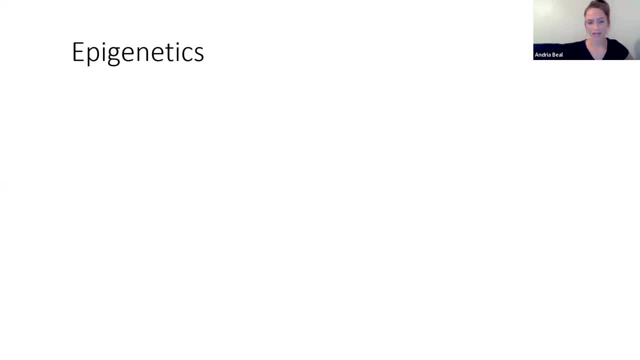 get to go over to Bimini, although you'll see where I sourced my samples from in a minute, so let me jump right in. In case epigenetics is a new word for you, I'd love to explain a little bit more A few of them. it may have been a little while since we had some genetic. 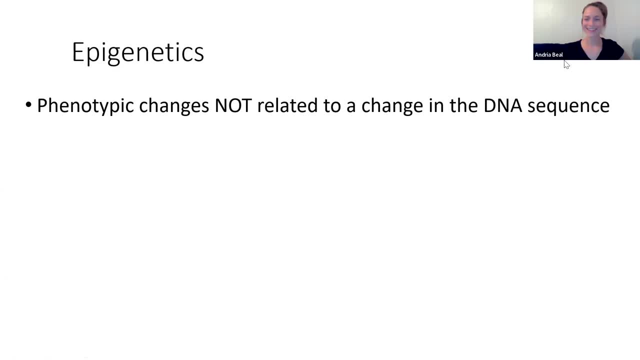 education, maybe since high school, some of them right. Okay, Please explain. Yes, absolutely So. with epigenetics we're talking about phenotypic changes, so what we physically see, although it's not related to a change in the DNA sequence. So we know our genes. 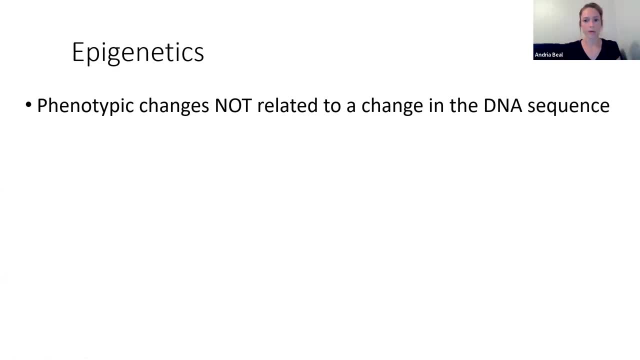 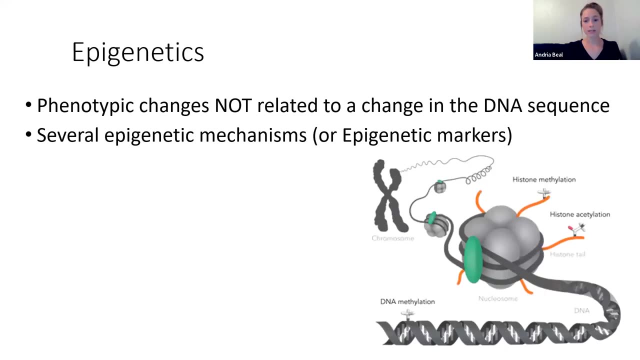 dictate these phenotypes that we see, but at the same time, there's a lot of influence from the environment going on. So there are actually several different epigenetic mechanisms out there, one that we'll get into what we're going to talk about today, but there's histones. 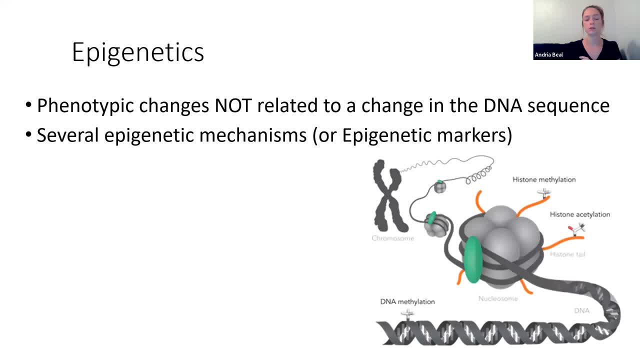 histone acetylation. there's modifications to these histones- that can happen. there's DNA methylation- all these things revolving around DNA, but don't worry, you don't need to know them. all These epigenetic markers are highly influenced by the environment. That's what makes them so great. 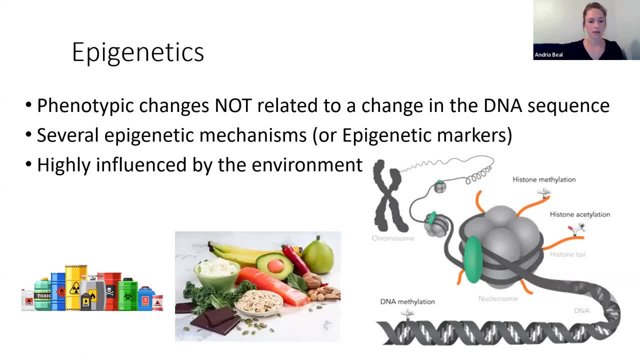 for environmental studies, as we'll get into. So your environment includes pollutants down to what you eat, whether you exercise or not, So they're very. epigenetics is very applicable to health for humans as well, And these epigenetic marks are potentially heritable, So they have big impacts when things happen in the environment and 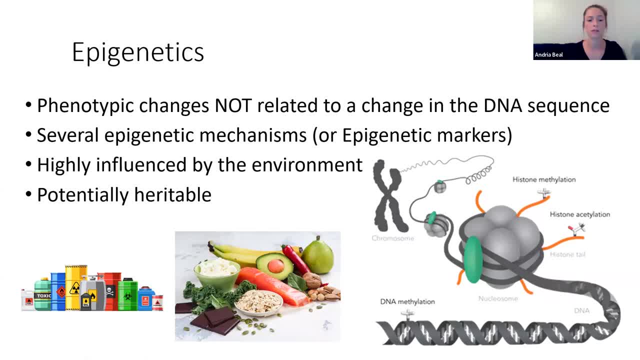 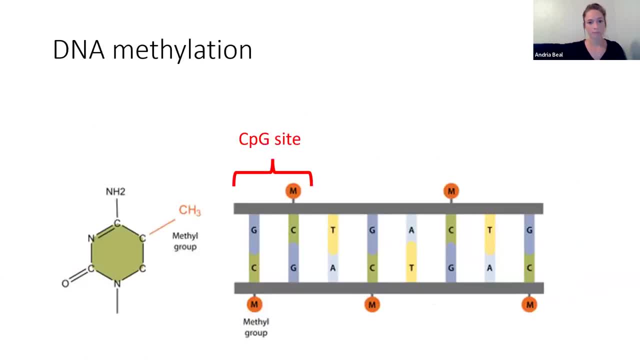 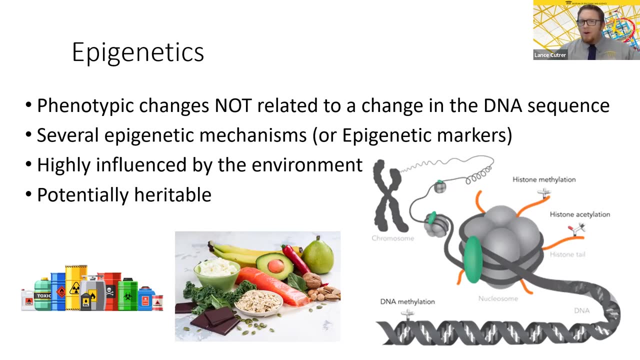 influence an organism, they can potentially be passed down to the next generation. So it's something we want to start studying and understanding. So- So-, Can I ask just one quick question? So so, basically, it's environmental factors can control what an individual looks like. 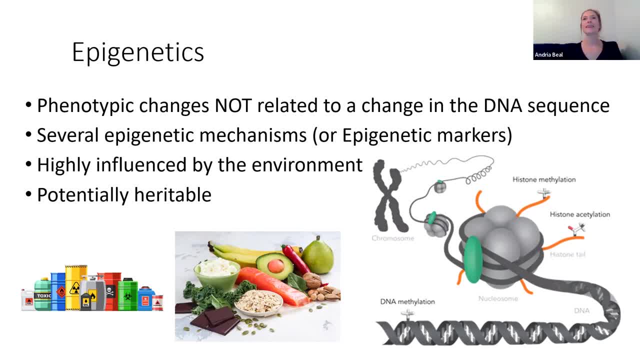 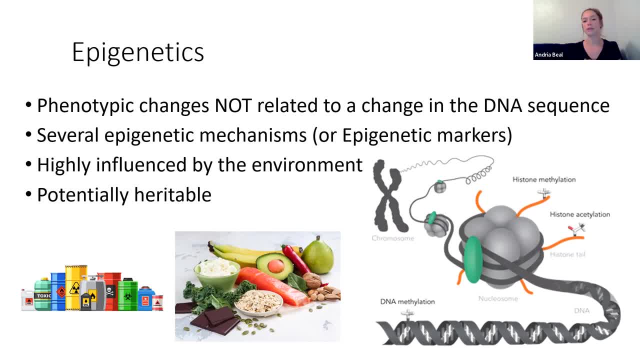 that mole to be in that spot. or you see identical twins with the exact same DNA And one of them develops cancer at a young age and the other never develops cancer. It's something in their environment that influences that. Because I think that's a really important point to make is a lot of people think of 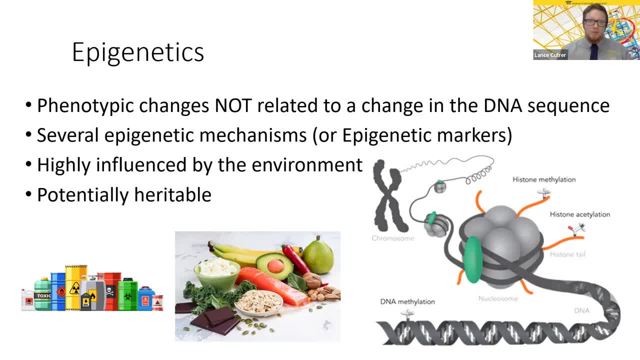 the environment and they think of, you know, pollution and its direct impacts on the on our outside of our body, maybe the inside of our body, with, you know, cancers and these kind of things, but to to affect, like the environment, that these animals and even us, 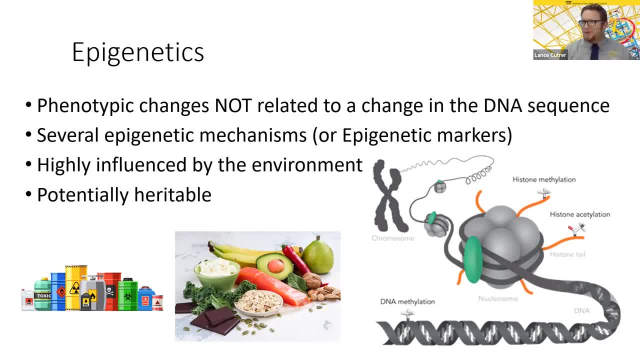 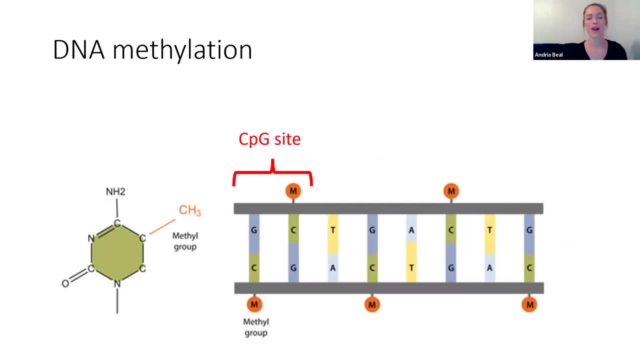 right, like you're saying, grow up in affects what they physically look like. it's i think i don't know. it's like i don't know. that's kind of amazing. it is amazing. that's why i love studying epigenetics. it's just, we'll get. we'll have a few more examples coming up for how this might happen. so one, so the. 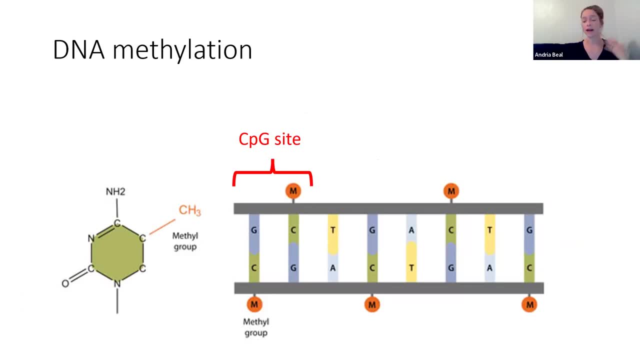 epigenetic molecule that we're going to talk about today, and the one that has been studied the most, is dna methylation, and so this is a methyl group that attaches to the outside of the dna, and in vertebrates it's most often occurring at a cytosine, so a c in the dna sequence, and it's 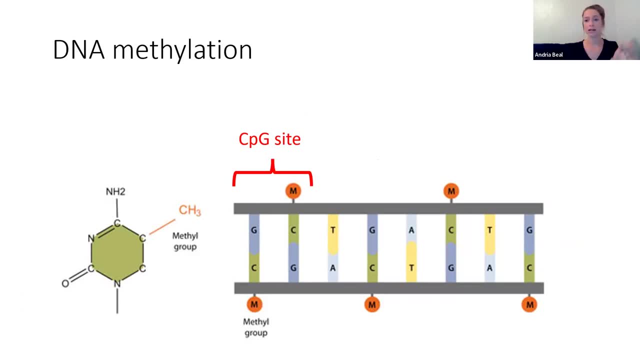 often next to a g, so we call that a cpg site, a cytosine next to a guanine, and so you'll hear me like to explain that. so when i'm referring to it later, you're not like whoa, um, so in vertebrate. 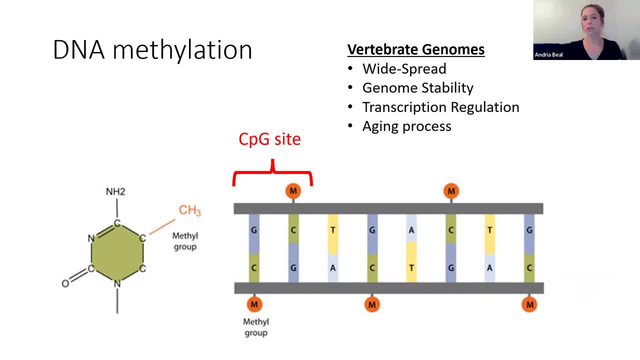 genomes. um, these marks are widespread across the genome. they help stabilize the genome, they work in uh transcription regulation and that's what genes get turned on and off, and they play a major role in the aging process. um, i always like to mention that because i'm all about age stuff. 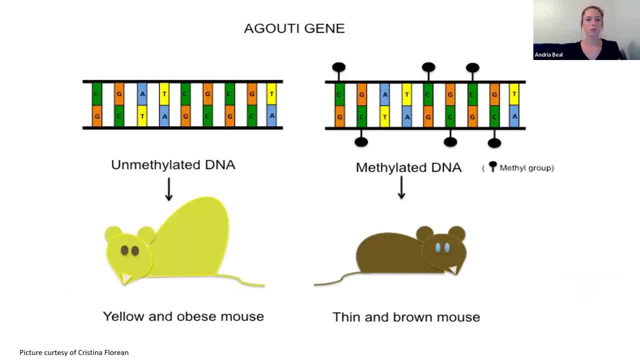 um, a great example of how dna methylation works is the agouti gene in mice. So this is one of these classic examples that has been around. So in mice when the agouti gene has methylation, you see a thin brown mouse on the. 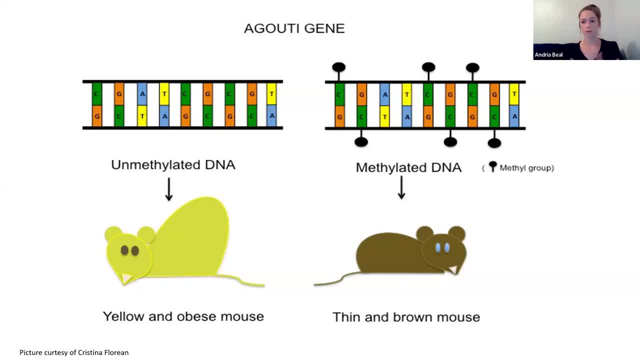 right over here. when it's present- And this is a normal phenotype for a mouse- If it's not present, on the agouti gene we see this yellow obese mouse, this phenotypically diseased mouse, over here, And what's really amazing about this is whether or not that DNA methylation is present. 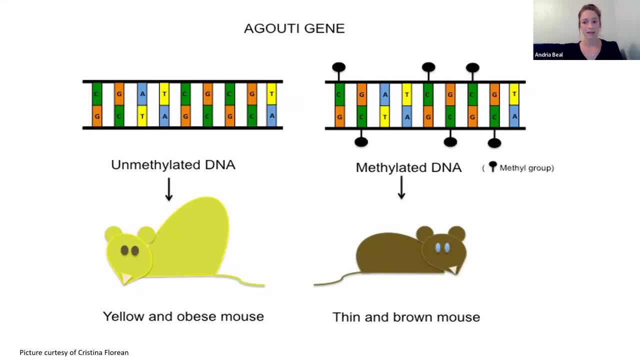 on the agouti gene is influenced by the mother's diet. If she was exposed to certain chemicals while she was pregnant, this determines whether or not this DNA methylation will be present and how her offspring will fare. So so so let me I just want to make sure I'm understanding correctly. So the in the slide. 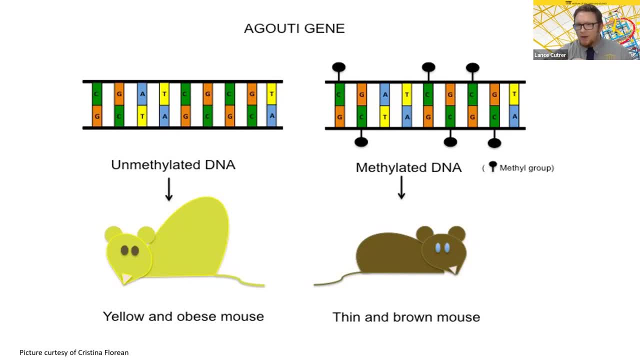 here. so it shows the, the amino acids of a DNA sequence, right? The adenine, cytosine, guanine, right I mean? so this is what a DNA sequence is made of. So if you put that methyl group in certain spots not affecting the DNA structure, the DNA is the same. You just add. 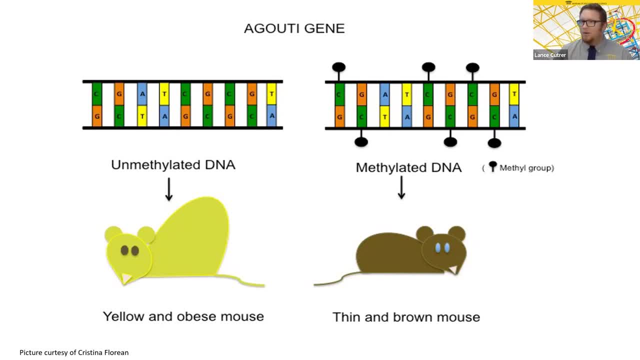 these little spots to the outside of it, It changes what they look like. Yes, Okay, Absolutely, Yep, And so essentially, it's turning off this agouti gene, or turning on this agouti gene, And so you see a different phenotype. 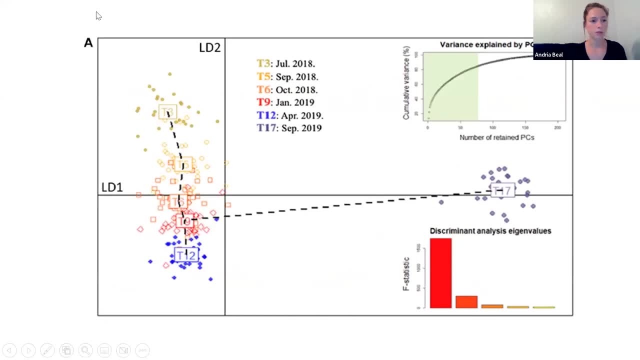 And then, with these methylation marks, we also see a change in the pattern of the overall across the genome in relation to things like seasons. This is a colleague of mine, I believe, who did a study on on coral and they saw this pattern change. 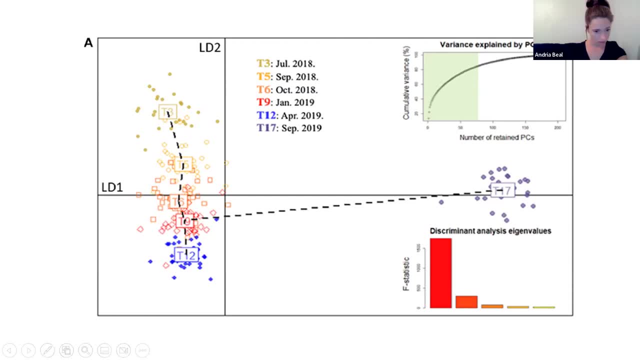 Let me see There we go. Let's have a laser pointer on here, So we see this pattern change. So here's one group that was sampled in July, and then we see September, October and so forth, And we just see this gradual change and it's correlating to the 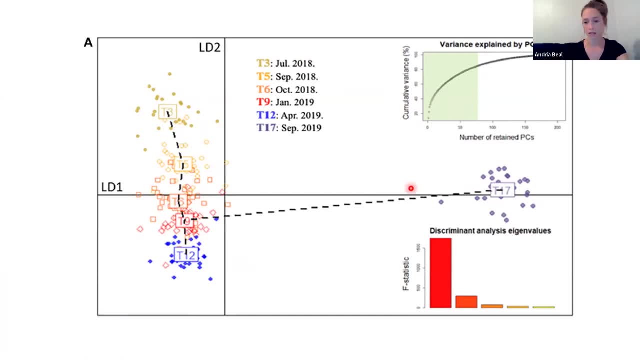 season that it was, you know, in the past. And so we see a change in the pattern of the overall samples in and then actually over here. this drastic change was- I believe it was- a hurricane, so we also see major disturbances cause this big change in these patterns as well. 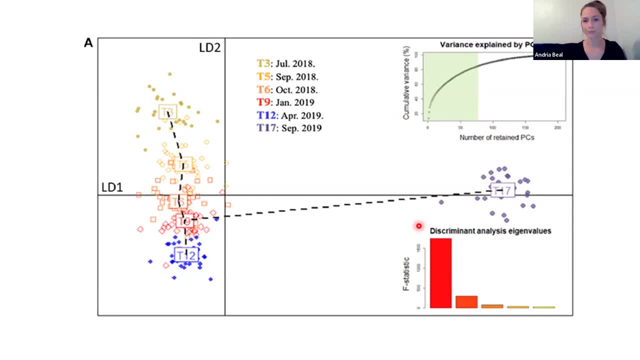 and this is just broad pattern changes. so with that we're going to get into a little bit more about the actual project that I did. this particular study that I have up here with the seasons and this hurricane event that occurred, is some of the back background research that helps spur the questions I had for this upcoming project. 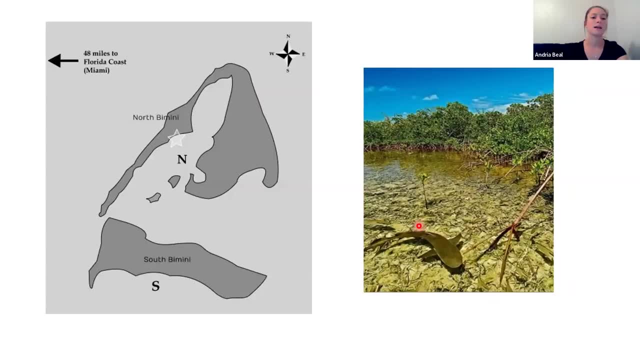 so with my project we were looking at a disturbance that happened in Bimini, Bahamas, and that this is Bimini here, a small bohemian island off the coast of the Florida, and our focus is on the lemon sharks there, and this is a lemon shark nursery, one of 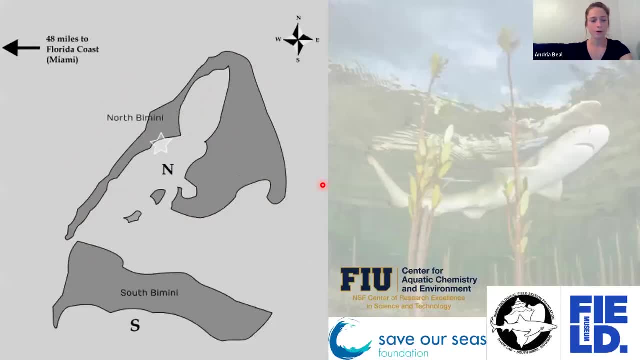 the biggest ones, and so with lemon sharks, when they're young they keep really small home ranges. so with that we can consider even within this small island different nurseries that are isolated from one another. so we have North Bimini in the north nursery here, and then we have 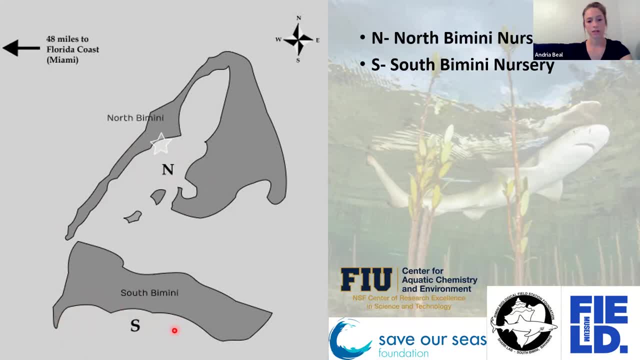 South Bimini in the southern nursery down here, and so these juvenile lemon sharks. they will stay within their respective nurseries to about three years of age, so that allows us to treat these as isolated groups, and what's interesting is that this major dredging event happened in. 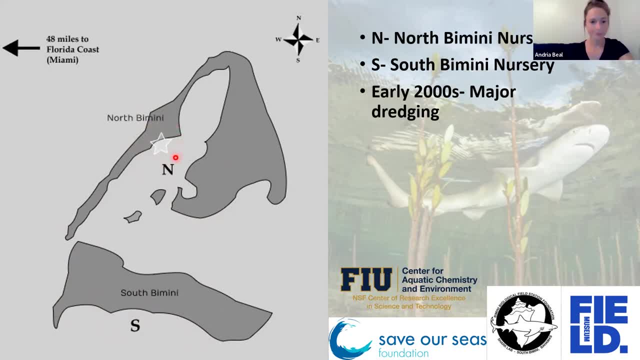 the early 2000s where this white star is here, and this was a dredging event of done by a resorts world, Bimini. it's a casino that came into the area and they were dredging to allow for really big ships to come into the marina, to come stay and visit their 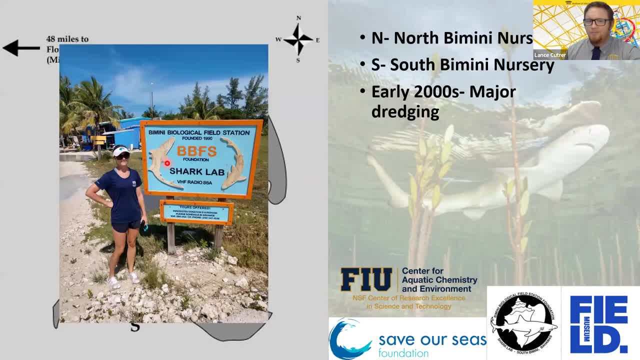 resort, and so in Bimini and South Bimini actually there's the Bimini biological field station where they've been studying these sharks since the early 90s, and so they have this archive of all the sampling they've been doing. so they've been sampling since the late 90s, so 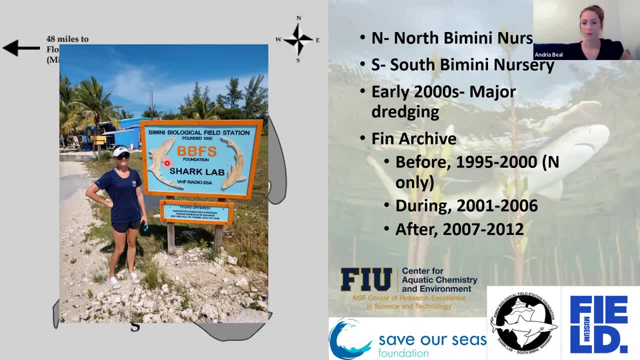 we were able to access this archive of samples to study what the DNA methylation pattern looked like, with this major event happening in the middle. so we have our get that out of the way. we have our before samples, which were sampled from 1995 to 2000, and then our 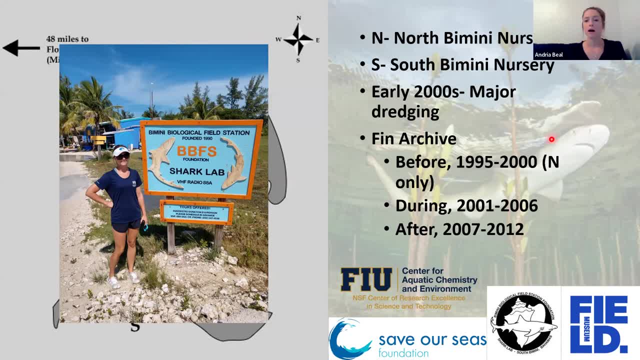 during this major dredging event is 2001 to 2006.. I think the bulk so dredging started in 01 and the most heavy dredging was actually done in like 04 and 05. and during this dredging event the researchers noticed that there was a loss of survivorship in the northern nursery where that dredging event was. 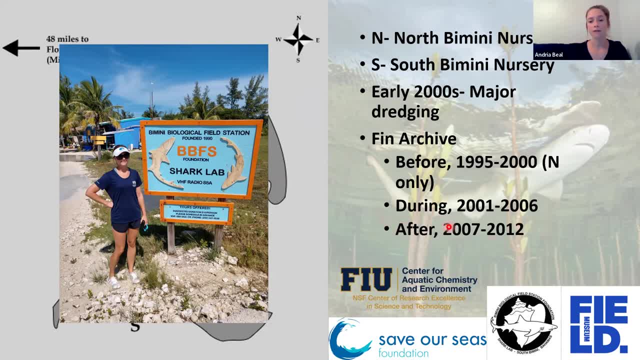 occurring. We also were able to get samples from after. a big caveat here with the study is that the before samples they only when they first start sampling in this area. they focused in that northern nursery, which is where most of the juvenile sharks are actually located, and so we were only able to get north. 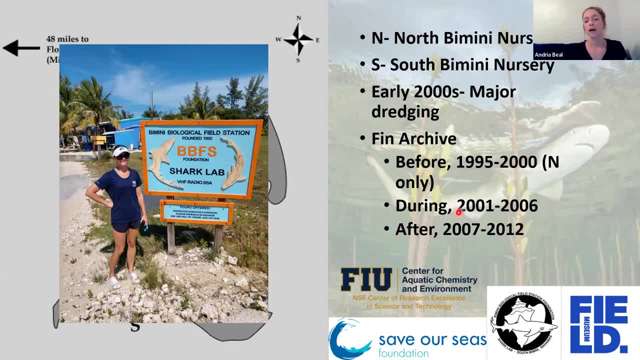 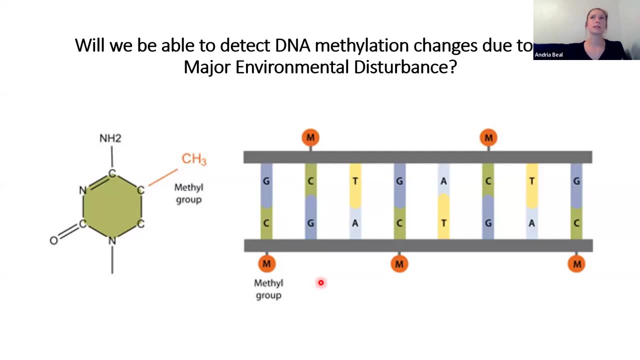 nursery samples for this before group, but then we had north and south nursery samples for during and north and south samples for the after group. And so the big question was really because epigenetics is a very new field of study and we can look specifically at certain genes, but with sharks we don't have very developed reference. 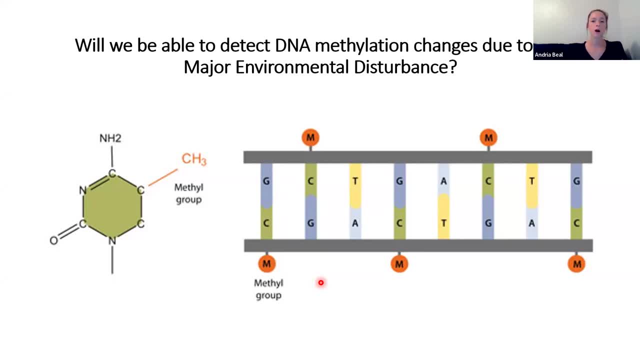 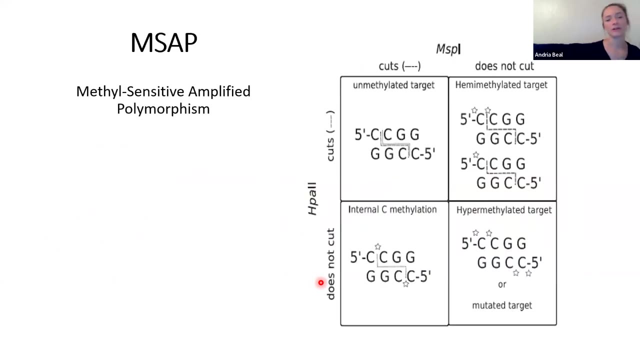 genomes. so it's very hard to do this. so we were thinking: let's look at the broad patterns of DNA methylation and how that change changes with this major disturbance. And so we used a technique. I'm sorry I'm getting a little technical here, but we use the technique MSAP, methyl, sensitive amplified polymorphism, And just. 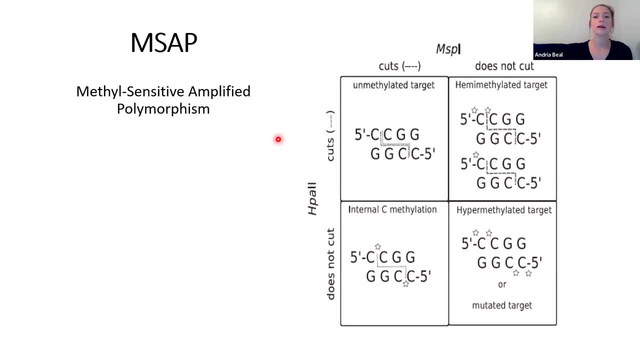 in case you're familiar with AFLP, it's very similar to that process, And what it is is we chop up the, we extract DNA, and then we chop up that genome with enzymes that specifically chop based on whether or not there is DNA methylation present, And so we get this cut pattern is what 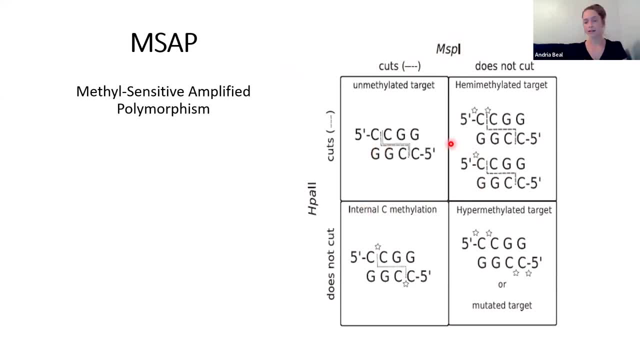 we end up seeing, which allows us to visualize that pattern of DNA methylation across the genome. And so, with this graphic over here we have the two enzymes We use: MSP1 and AFLP1.. And they both recognize the sequence CCGG, but they cut based on what kind of DNA. 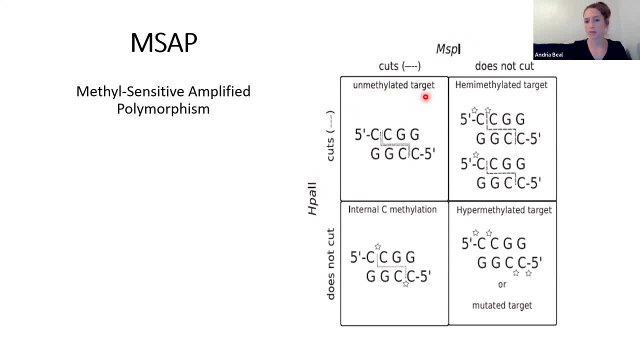 methylation is present or not present. So if it's an unmethylated target that comes along the DNA sequence, it's CCGG and there's no methylation present, Both of these enzymes are going to cut the DNA sequence there If there is hemimethylation present. so HPA1 and HPA2, and they both recognize the sequence CCGG, but they cut based on what kind of DNA methylation is present. So if it's an unmethylated target, so there is methylation on only one side. 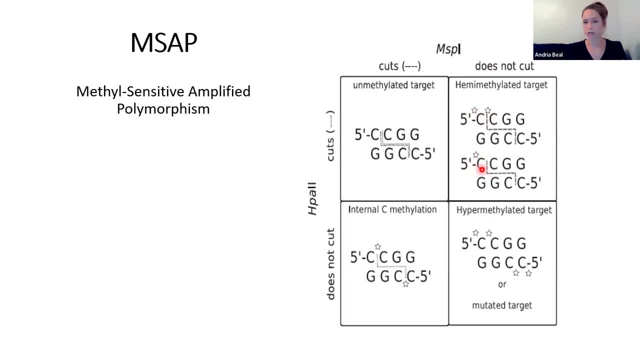 of this DNA sequence, whether it's both Cs or just one, we're going to see a cut by HPA2, but not by MSP1. And then if there is, say, hypermethylation down in this quadrant, we see neither of them cut. 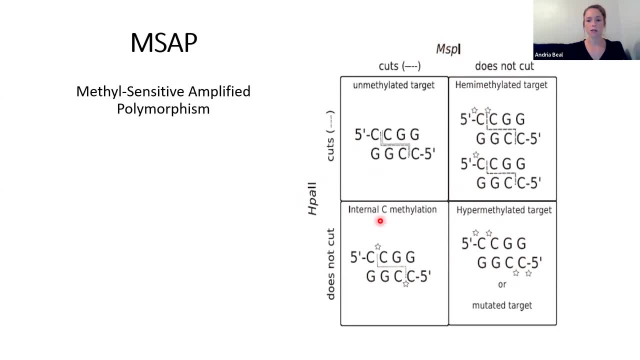 And then if we're only seeing a cut by MSP1, but not by HPA2,, then we have internal C methylation And the stars are represented. So if we were to run this DNA out on a gel, we would see marks on the gel for if there was a cut or not a cut present. 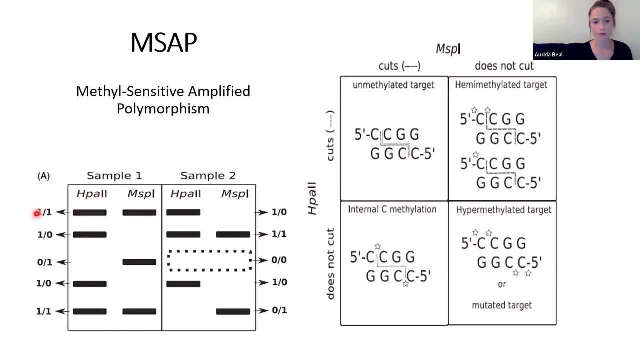 So here we see that both of them cut in this first one. So here's one sample, Here's another sample and you can compare them right. So on this sample we have two cuts. So two cuts is an unmethylated target. So if we were to run this DNA out on a gel, we would see marks on the gel for if there was a cut or not a cut present. 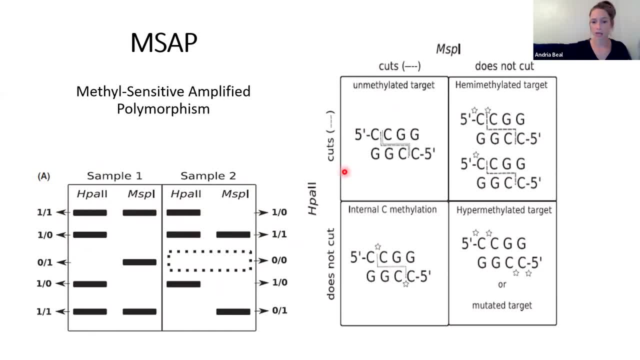 So here we see that both of them cut in this first one. So here's one sample. Here's another sample. We have two cuts, So two cuts are an unmethylated target here Versus this one. we have a cut by HPA but not by MSP, So we have a hemimethylated target right here. 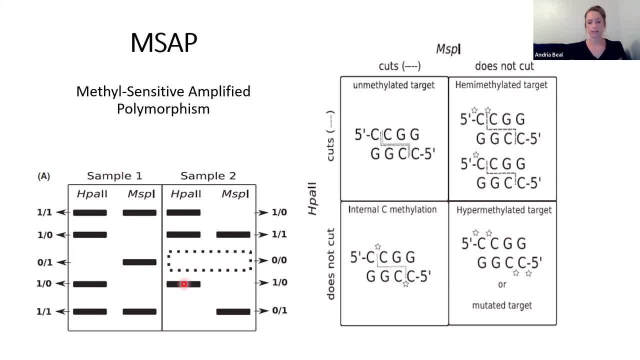 And so we can compare the patterns between sample one and sample two and see how they differ. And so this could be say: sample one is the before group, sample two is the during group, and we can compare those two patterns. So that's essentially what we did for our study. 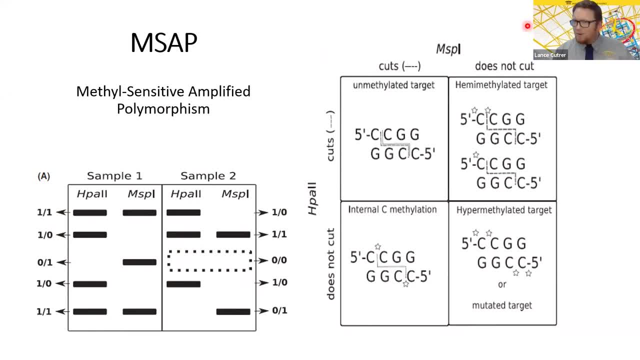 All right. So I just want to make sure I understand right. Is that okay? Absolutely So. when you have a DNA sequence, the DNA sequence gets read. Your body, the cell, reads that DNA sequence and that instructions of what to do, right? 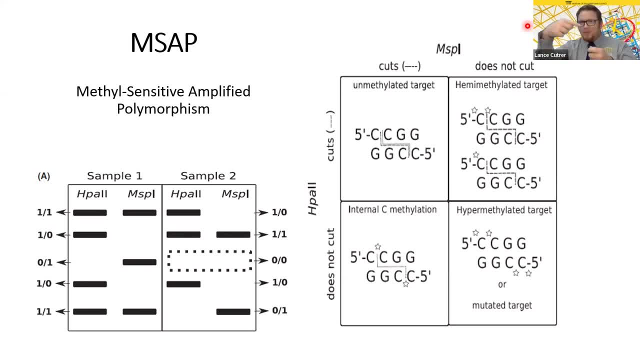 Using enzymes, right. So the enzymes run down the DNA sequence and it spits out instructions that go off to the cells and it spits out RNA, And then that RNA gets translated by the cell to do something, to change the cell in a certain 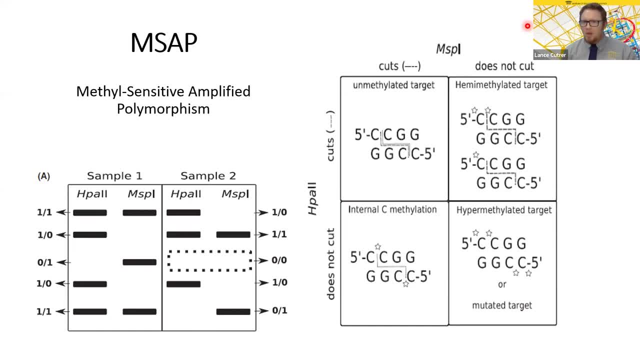 way, or to make a protein right. So by running this, the MSPL and the HPA-LL enzyme down right, It would cut the DNA sequence at certain points right, And when it did that, it made marks in your gel. 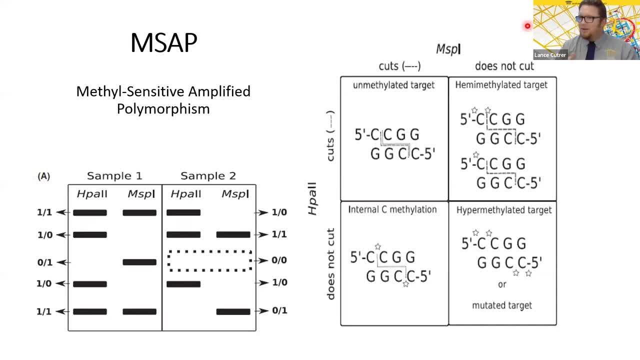 So it's like a physical thing that you see. Yeah, it's fragmenting the DNA, And so this on this gel: we can run DNA out on a gel and visualize it and see these fragments that we've created. Right, Okay? 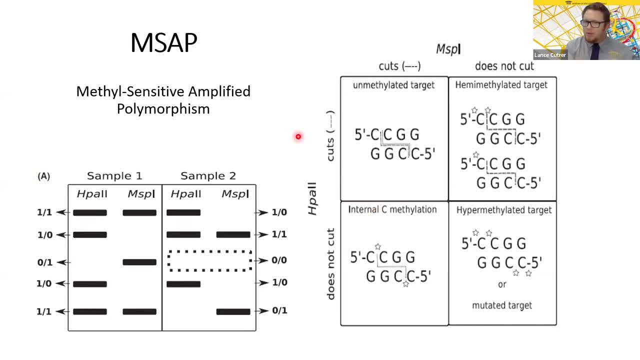 And so so, from doing that, you can take your samples from before the dredging and then after the dredging and then see if that those methyl groups that cause the individual to look different are present. right, Okay, That makes sense to me. 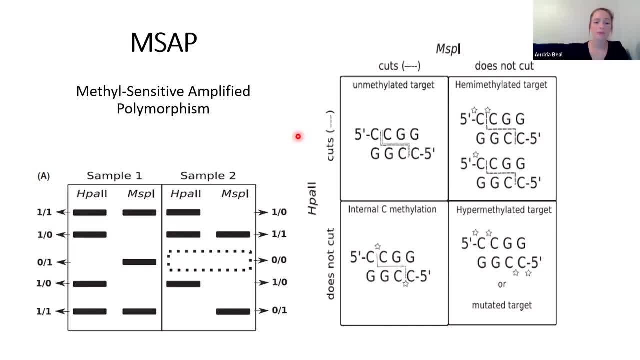 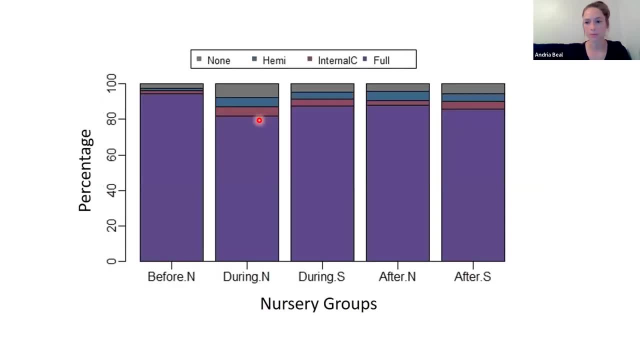 I understand, Thank you, Yeah, So we, we fragment the DNA and we check out. you know where there were cuts and not cuts, And actually. so this next slide here might help visualize what we, what we get from this DNA pattern. 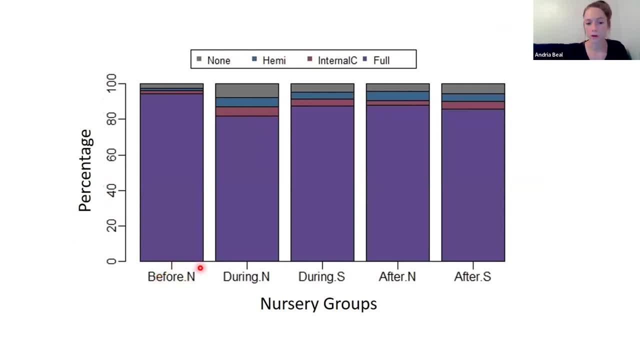 Um. so here we see that the before north group- um, they had a lot of fully methylated um DNA, So a lot of fragments, So fully methylated. we had a lot of cuts. versus the during north group, we saw a lot. 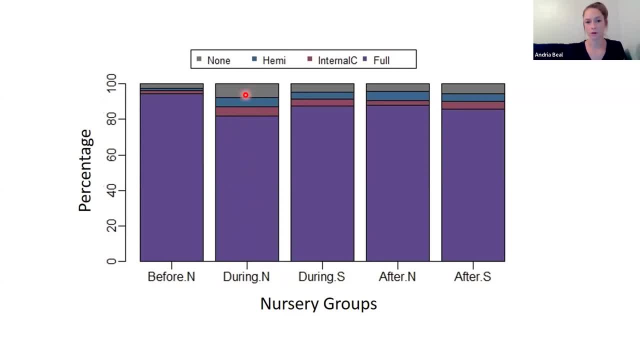 less fully methylated and more of these other groups. So a lot of no methylation, a lot of hemi and an internal C. So there was a lot less methylation present And this is our um, our exposed group that was directly closest to the dredging event. 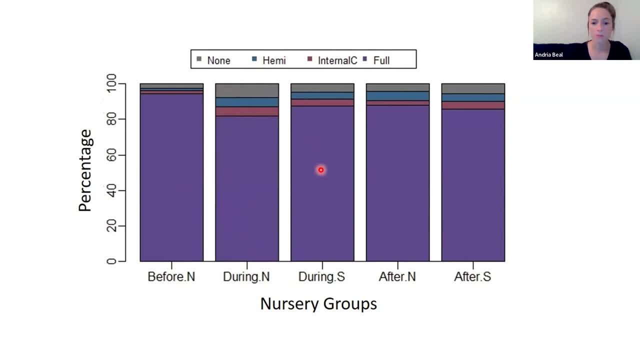 that we were looking at. Then we have um, the during the dredging event time, but in the southern nursery. so our control group, Um and we see that they have more fully methylated DNA, And then our after north and south. they're actually quite similar to one another. 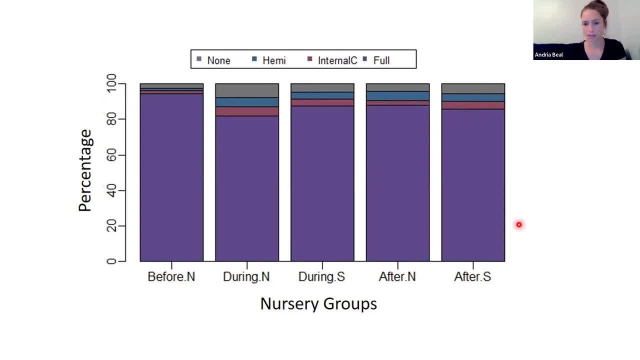 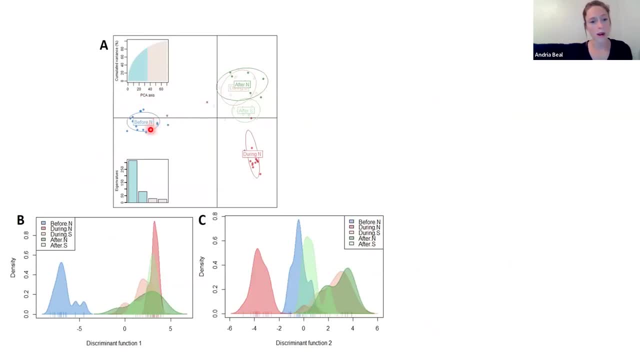 Um, and- and let's see, this is a better way to look at this now- Um, so here's an AAPC graph um, where we plot out the, where we plot out the points based on that DNA methylation pattern. 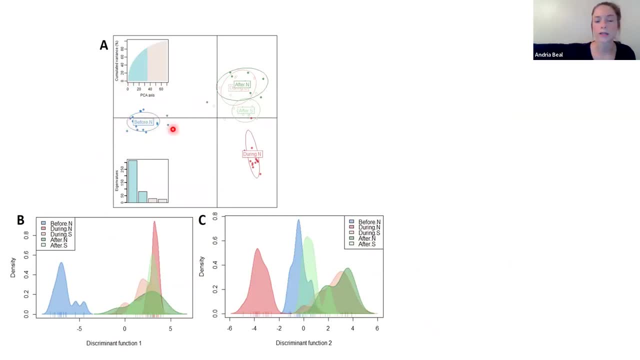 Um, and you can see that between any two points it's describing how similar or dissimilar it is to another point. And so here we have our before north group, which is much different than all other groups. Um, and here's where we realize it's really disappointing to not have that south nursery. 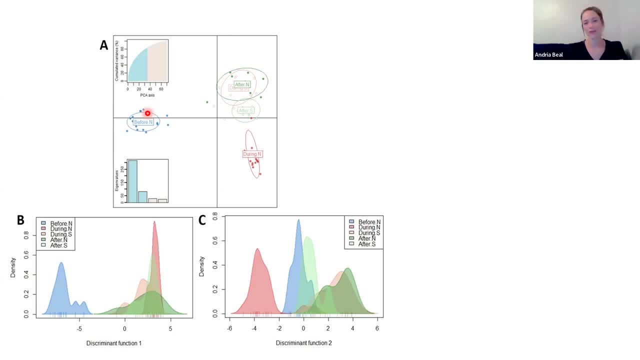 group in the before time to see what it looks like, And that's just one thing that we can't control. Control for in this opportunistic kind of study, Um, but we see that before north is very different from all the other groups. but then we also see that our exposed group- 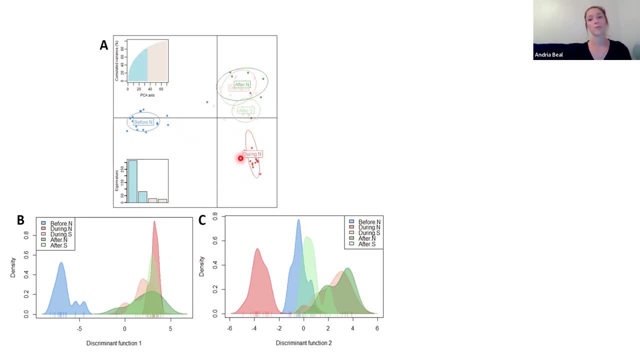 the during north group is much different than all groups as well. So, um, then we have the after north, after south and the during south are all pretty similar in grouping together. So, um, these graphs down here, B and C, we're going to hone in on the different axes. 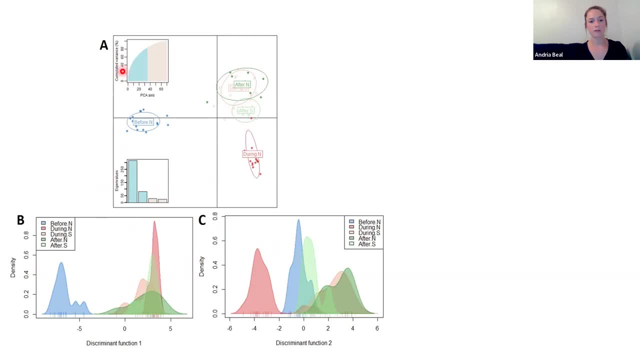 So B is as if you're looking at that, this uh Y axis across it And, oh, I'm sorry, looking at the X axis, sorry this way. And so you see this before: north group: much different from the other groups, right. 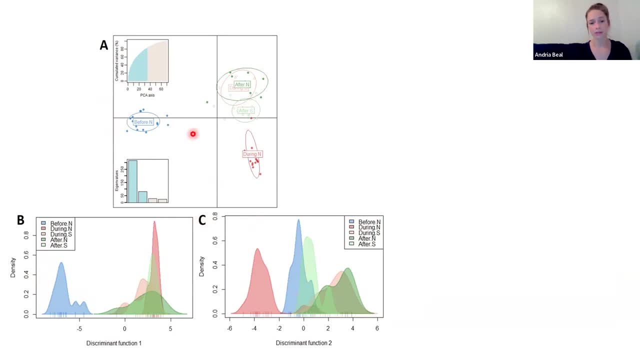 And then C is as if we're looking at the Y axis. So this way- and that's where you can see that our during north, our exposed group, is um, separating out from all other groups over here in there, And this is in their DNA methylation pattern. 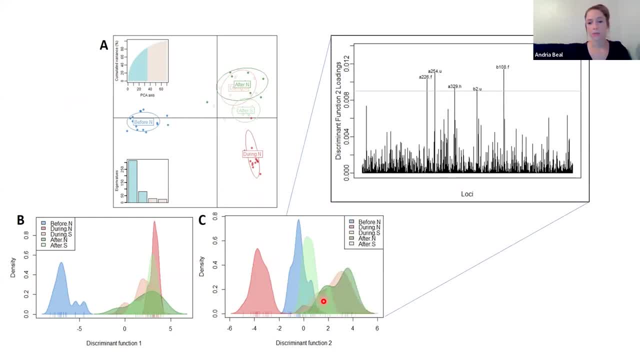 What we can do is look even deeper, And so this is the actual fragments, individual fragments that we we got from our analysis, and you can see which fragments are driving this differentiation, And so this is exciting for future studies. Um, this is where, if we had good 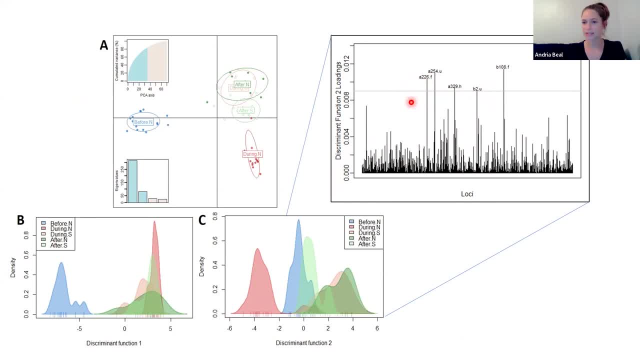 Reference genomes. we could go in and pull these fragments and actually sequence and see what parts of the genome were affected by this dredging event. In this instance we don't have good reference genome, So it's not worth us going and trying to sequence, um, and doing all that extra work to try and figure out what's really. what's the effect of this dredging event upon the actual shark? 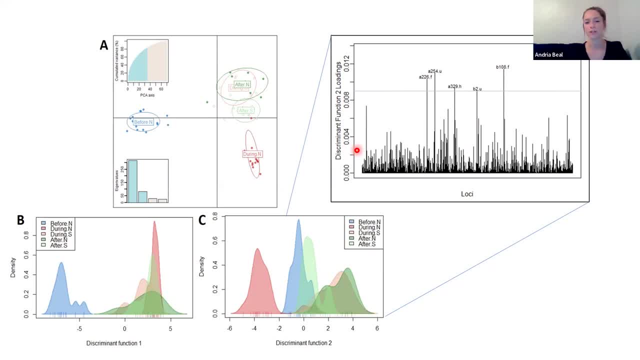 Um, but this is something that we can come back later, once we have those reference Genomes, um, and actually do future work and find out. So what happened to a shark when the dredging event happens and their environments turned upside down, like what physically affects them? 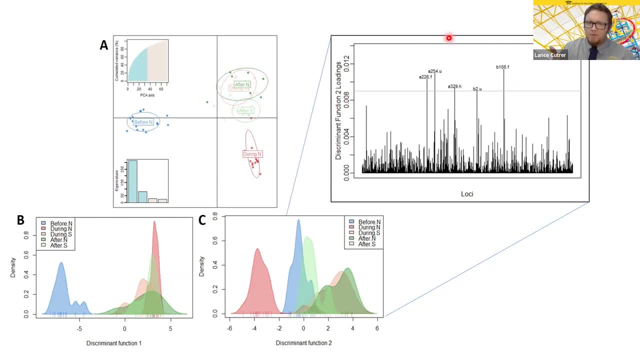 That's really cool. So so the, the graphs, just to interpret them a little bit. So the the, the graph that's labeled age is the. the further apart they, these, these groupings are, these samples are from one another, the more different they are. 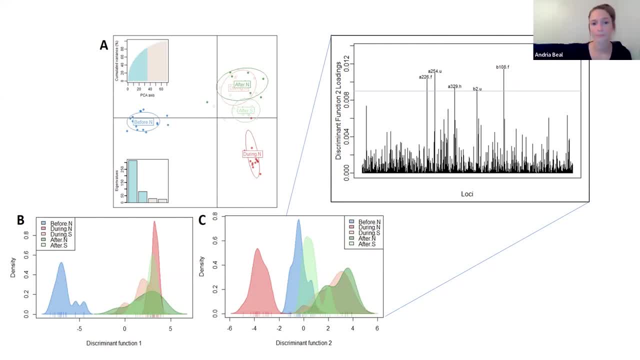 The right, So the the less. methyl is a uh um methylation. they have based on the ones before, So the further. the further they are apart in the graph, the more different they are. I get it. That's really cool. 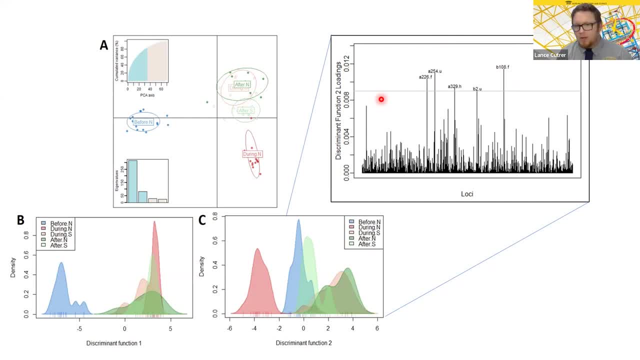 So, so, like. so you could say like for future studies. you could say um, oh, I want to. we know this dredging project is going to happen Like it happens in um, or maybe it's like a beach renourishment. 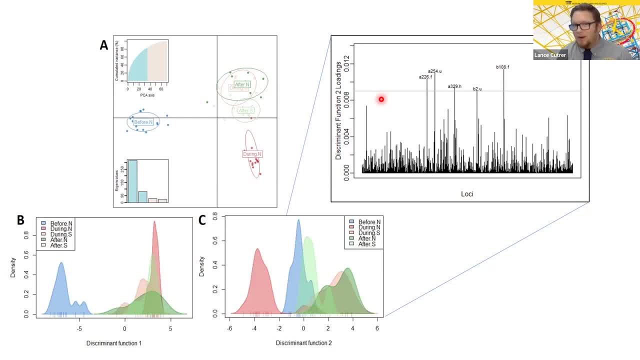 Situation off off our coast. here in Lincoln, Fort Lauderdale, We have that happen all the time. Um, sometimes they dredge to get the sand for it. Um, if we know that's going to happen, then maybe a researcher like yourself could then go ahead of time, maybe get some, get that foundational sample right before and then sample during and then after and see what that that effect is. 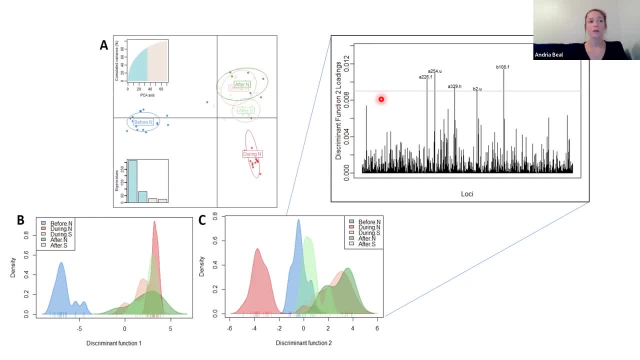 Right, That's really cool. Absolutely Yeah, And so actually something that I talked about a lot during my dissertation was the need for long-term study of epigenetic biomarkers, because you kind of need that baseline of what's normal. Um and, like I showed before, we know that seasons have an effect on this overall pattern. 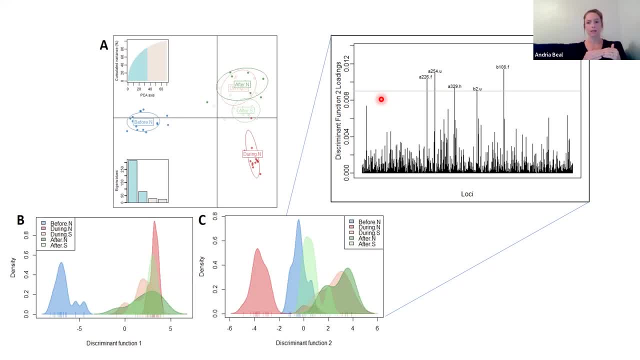 So we need to know what normal looks like in order to visualize what the disturbance is causing, Right, Um and so like. in this case here, unfortunately, we don't have before South samples, so we just have to take before North as the original normal right. 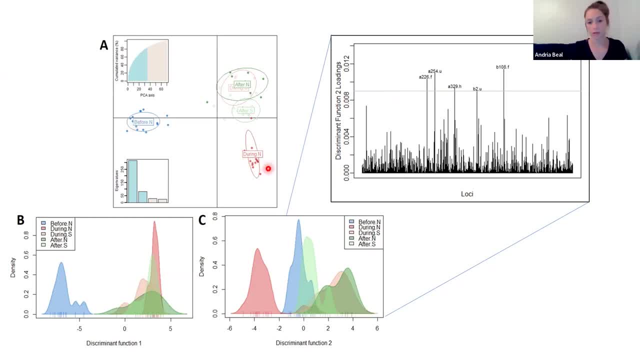 And then we see that there's this big change when the dredging event occurs here and we- and luckily we had during South samples and we see them over here, So we're going to assume that this is the new normal during the during timeframe. 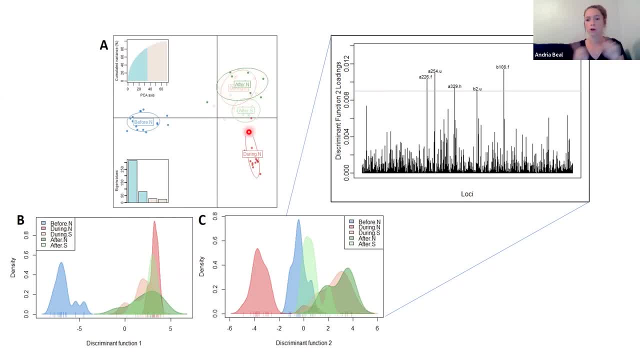 And it's very similar. We see the after North returning back to normal is how we interpret this. So, um, these baselines, they're really important and that's my big um. what I advocate for is that we need more money for conservation to go towards these long-term um studies that are out there. 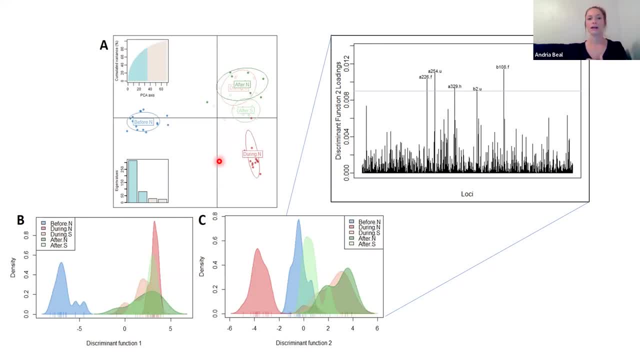 There's like a long-term study in the Everglades right And um. they're sampling and getting tissues all the time. Yeah, And it would be great to designate some of that money towards doing things like this, like the broad um epigenetic patterns. 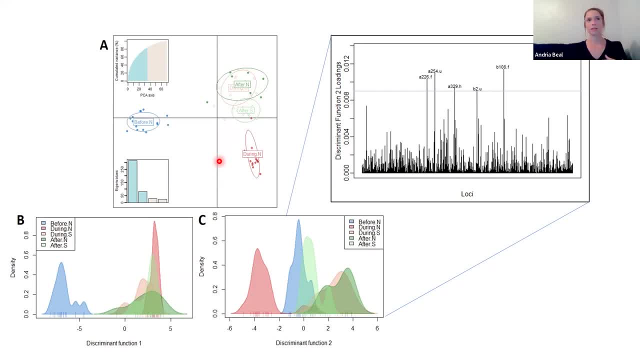 So that way, when we go back through or something major happens, we have- oh, I don't know- a spill or something, you know a chemical spill, and we want to figure out what's going on. We have that normal baseline to look at and see how things have changed since then and be able to correlate better to the different things in the environment that are changing. 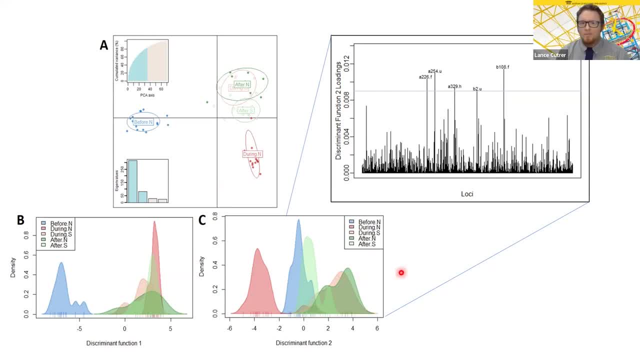 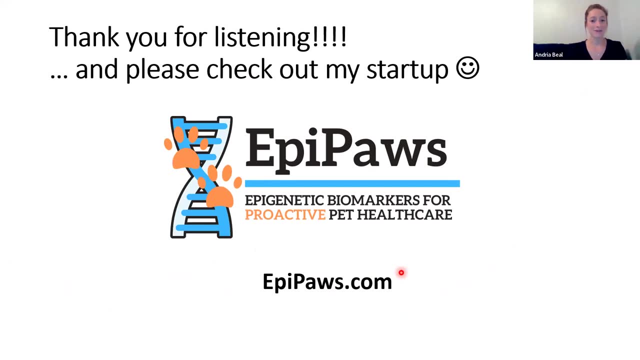 Yeah, that that totally makes sense, And so that's that's all I prepared for tonight, Um, but uh, thanks. Thank you everyone for listening And if you have any questions, we can chat some more, and I do my shameless pitch. 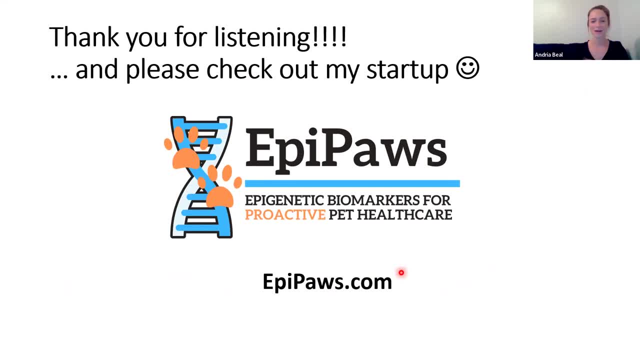 I'm a new graduate from my PhD and I started a company um EpiPaws, So please go check that out, especially if you have pets. uh, we're working to hopefully design some epigenetics- Yeah, Epigenetic biomarkers- that can help identify when disease is starting to develop. 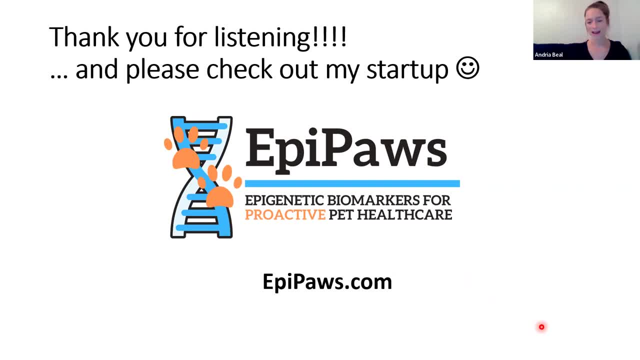 So that way we're more proactive and we can um get ahead of diseases and hopefully avoid some of them. Very nice, Um, very cool, All right. So, uh, I guess I have a question for you about, um, I guess, what? what are the physical changes? 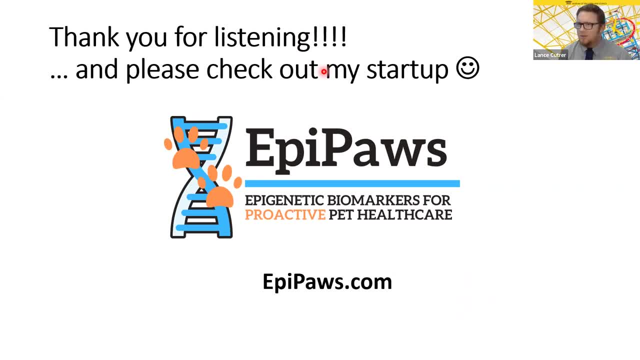 Can you see the physical, the phenotypical changes in the lemon Um? So in this, no, And so in this study we didn't physically see a change Um, they only noticed that there were. so, with all these um samplings they were doing, they did notice that the recaptures in that area during that um dredging event, um became less. So they were recapturing individuals less, And so that they took that as a survival And they did um, you know, um, um, um. there was a lot of um kind of like a canyon in the bay area that had a survivor ship that had been traveling, um, that lasted in the bay for a long time. 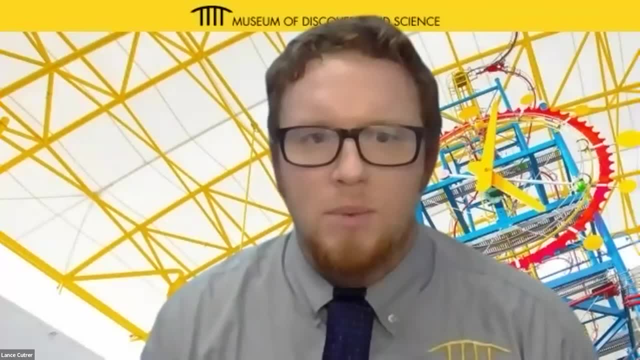 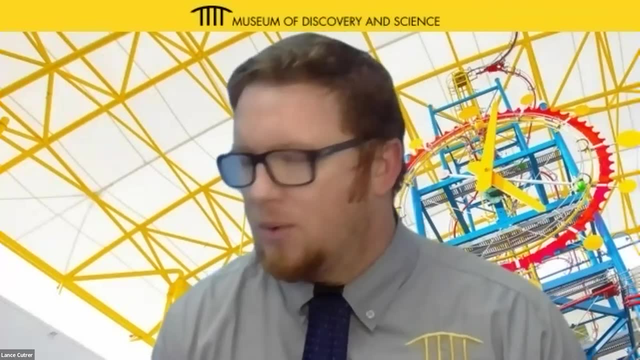 And um, there was, um, there was a lot of um, um, there had a survivor ship, but nobody had any survival ship that had ever had a survivor ship change. Um, there was a lot of other organisms in the bay area there that also um had a survivor ship decline during that dredging event. 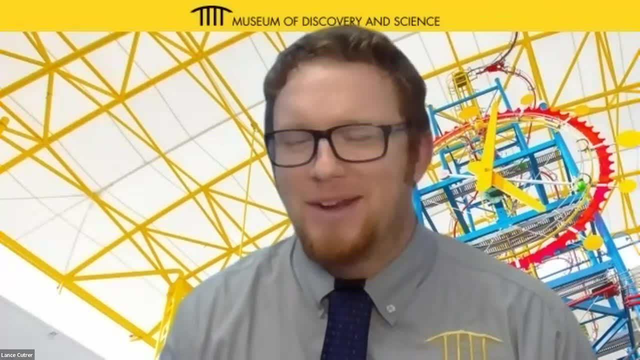 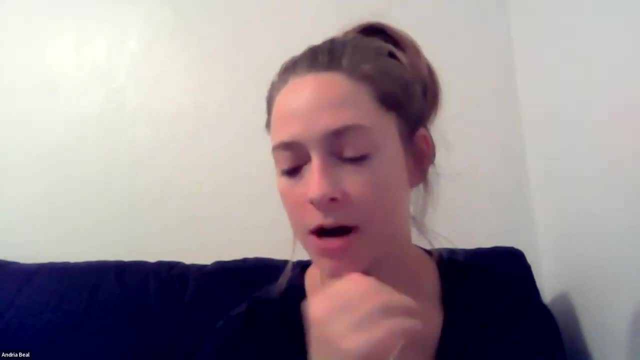 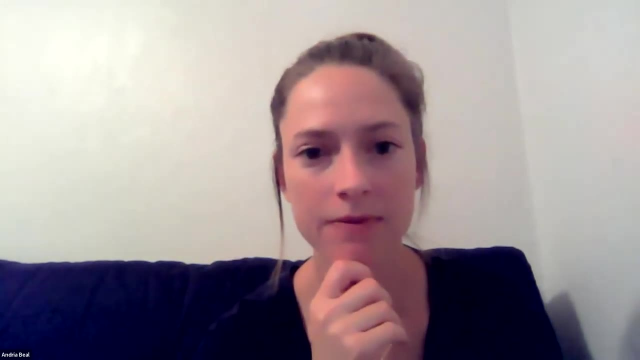 Okay, So some Something happened that allowed them to not survive As well, Right, So okay, Yeah, So it wasn't so much like that, And I will say that we did. there was a hypothesis that perhaps during that dredging event, trace metals were probably introduced into the environment. 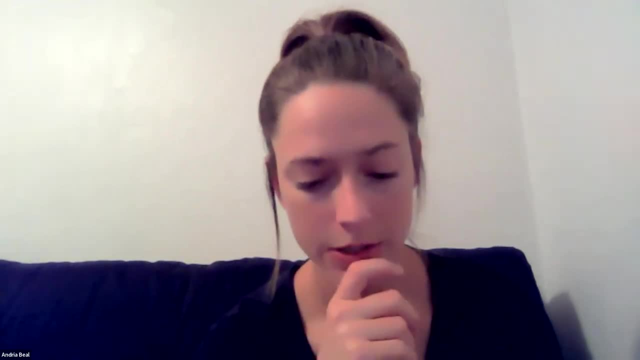 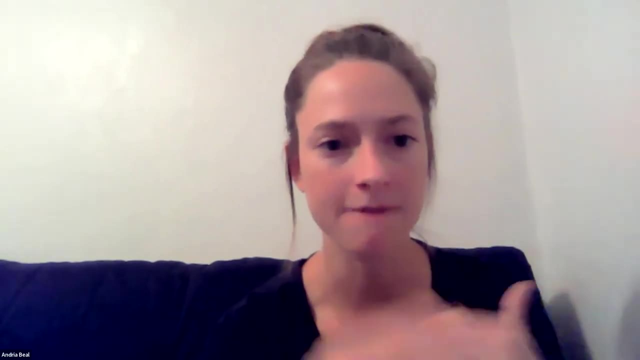 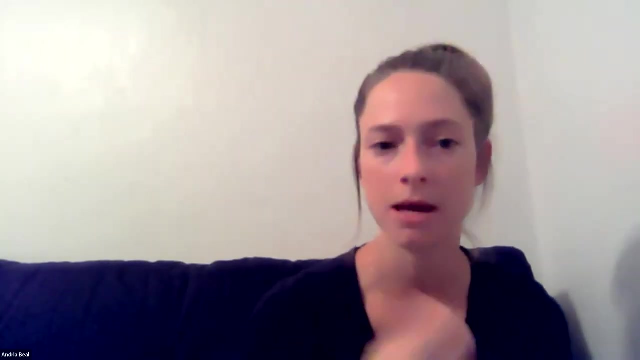 And so we did. we were working with thin clips, And so thin clips aren't the ideal tissue to look at trace metals. that would be changing that fast pace. Um, you'd actually want to look at something more like I don't know, something that is directly processing metals that might encounter maybe the liver, kidney or something like that. 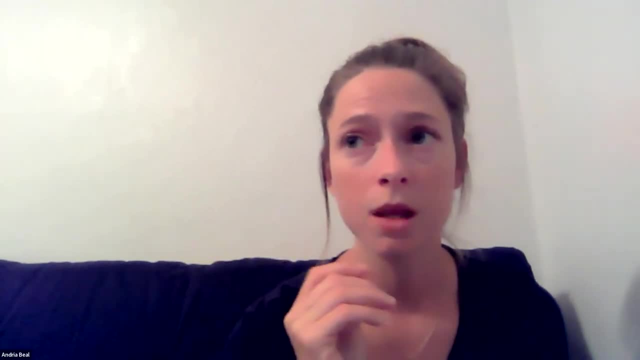 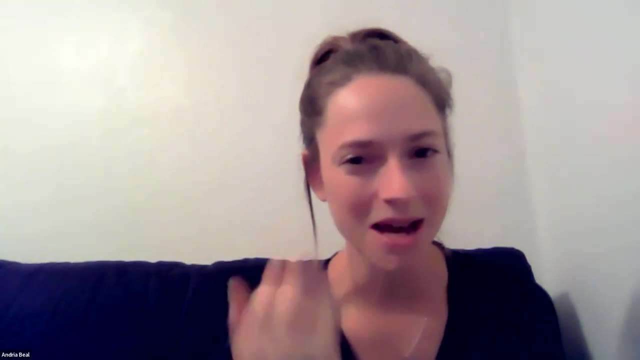 But since it was thin tissue, um, we did go ahead and look at a couple of metals, but we didn't find anything interesting with metals. But at the same time, working with thin clips didn't really expect to catch. you know, if they're be able to see that, 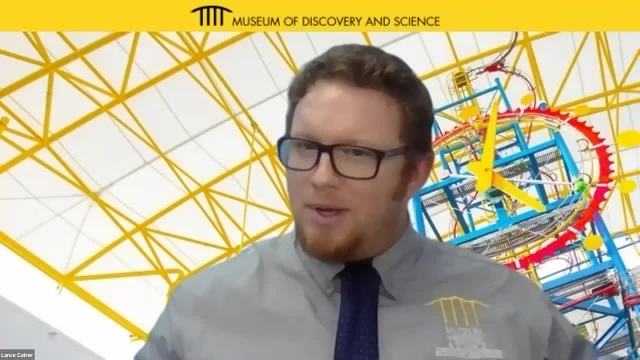 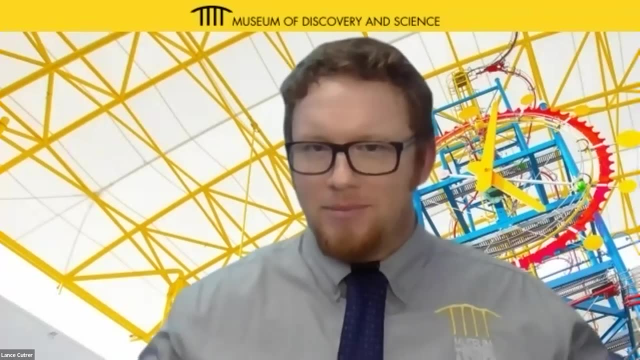 Right, Could you? could you explain that process a little bit Like so. So how did you collect the samples that I mean, and how old I mean it can these weren't adult lemon sharks that can get 12 feet long, I would assume, right? 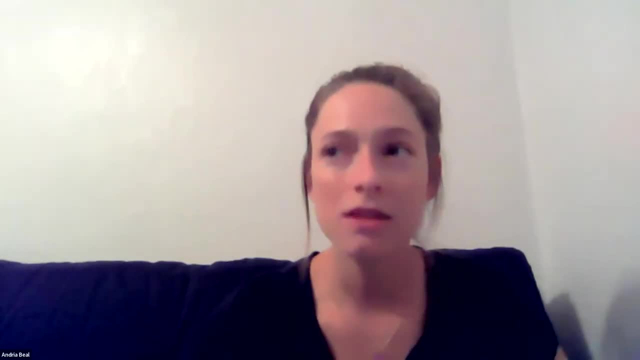 They're? they're juveniles, I would assume Yes, Um. so all the sharks in the study were three years or less. Um, I think a majority of them were um one year olds. actually, that was our majority. uh was one year olds. 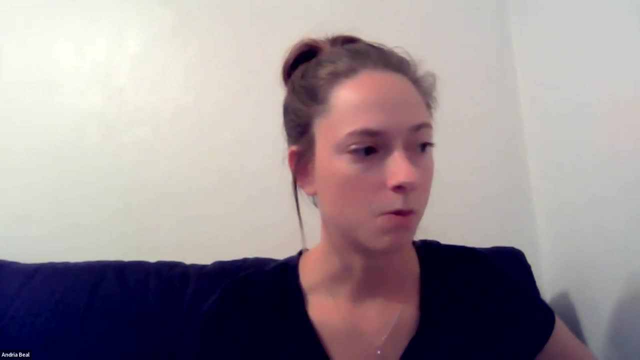 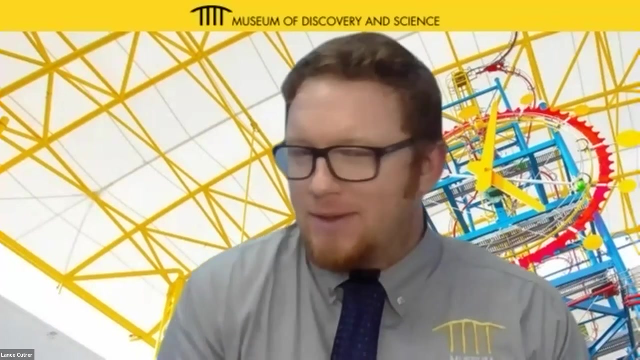 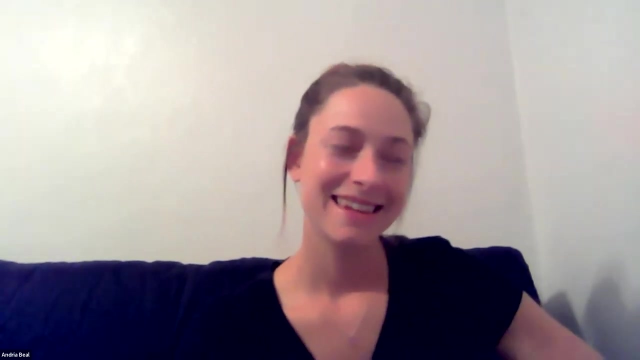 Um and Um, one and two year olds. actually there was a lot of two year olds, um and oh. I just lost my train of thought. I was gonna say something else. Um Yeah, just like explain how, how did you capture the sharks? how did you take the samples? like what? how did that tell us? tell us the story of going out into the mangroves and looking for lemon, human out lemon sharks. 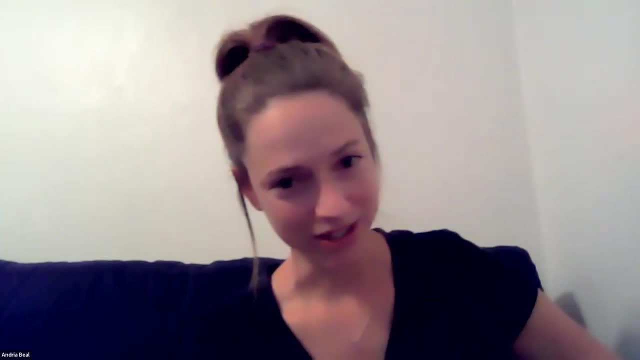 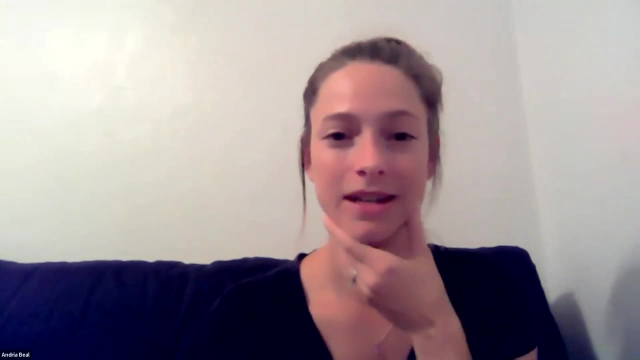 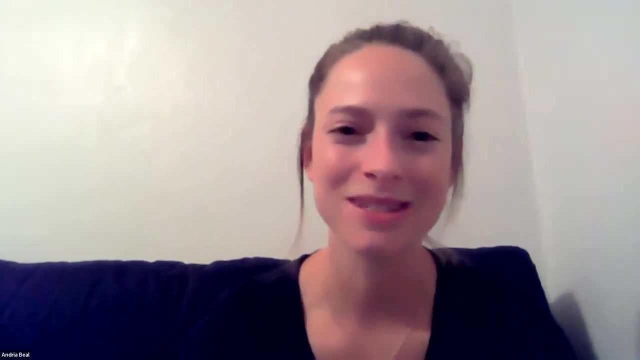 Well, unfortunately I did not get to go sample the sharks. That would be an exciting story, But um so, Uh, these were all archive samples and the Bimini Shark Lab. they had the honor of getting to get, get all those cool samples. um, all the sampling stories belong to them. 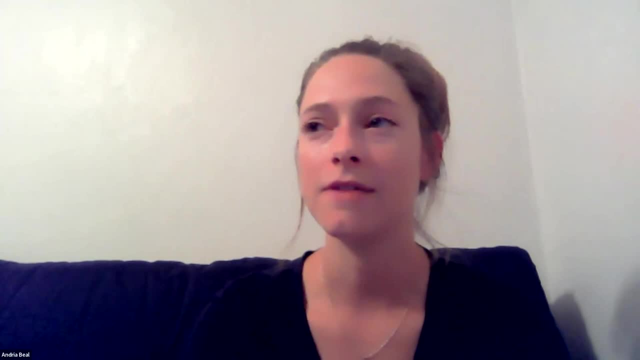 Um, but a lot of their. I will say that a lot of their um sampling occurs at night and they set up nets and catch them and they sample them all in like a couple of nights, like back to back. 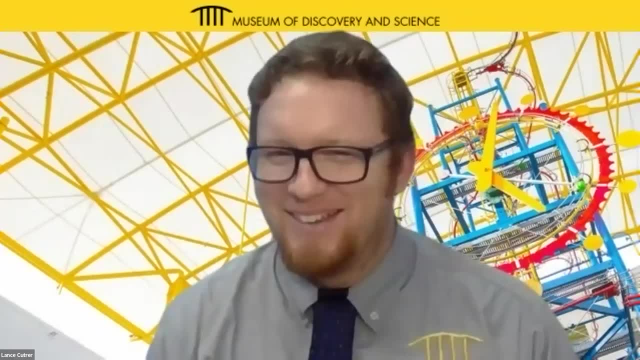 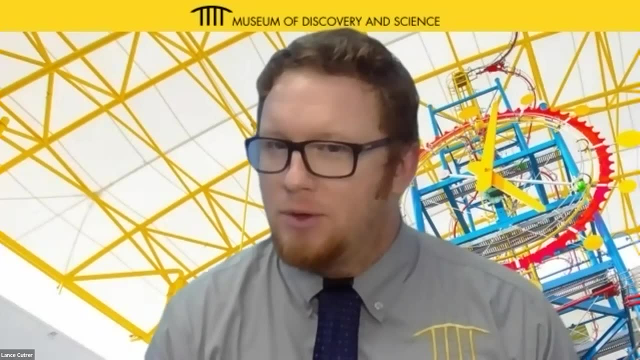 Um, but I didn't get to participate, That's okay, All right, So that's interesting. So so they'll go out at night, capture the sharks, take a little piece of their fin and then, and then let them go, I would assume, right. 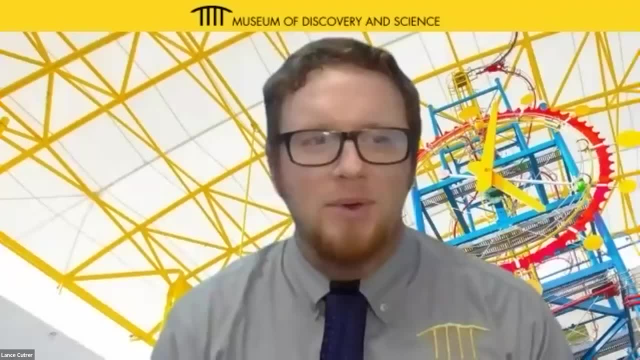 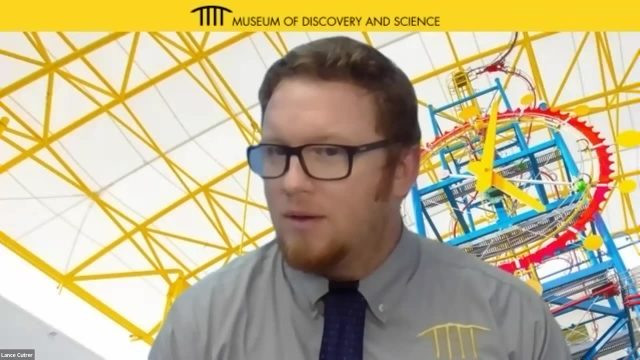 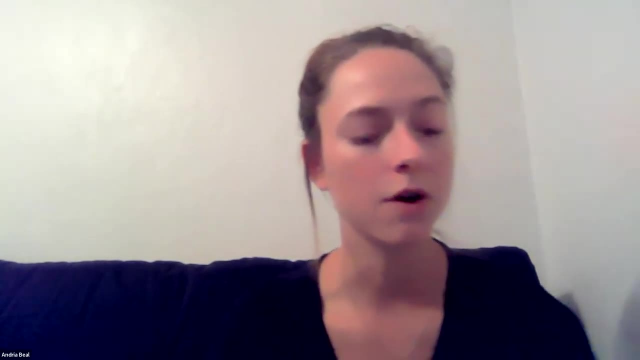 Yes, absolutely, Very nice. Okay, Has there been any other research like this? um, this epigenetic research done with any other species of shark that you know of? Um, yeah, there are a few studies. Um, there's been like an overall methylome of- I think it was- whale shark. 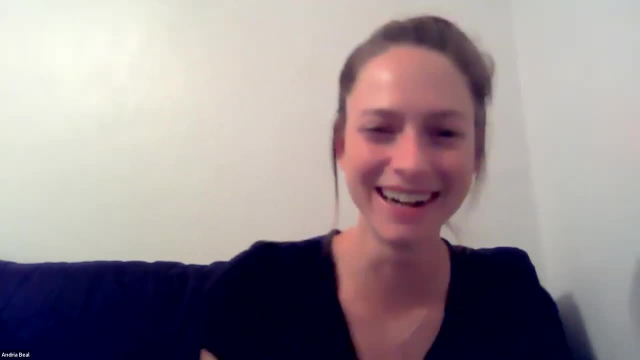 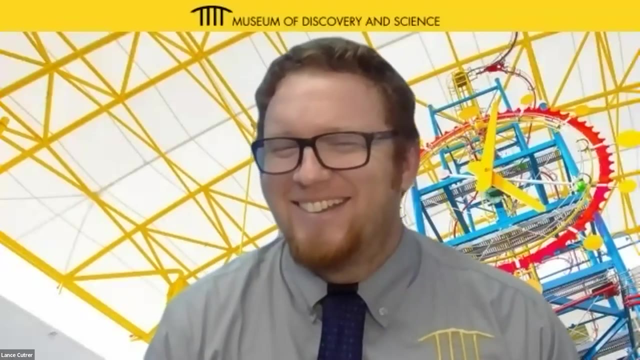 It's been gosh, it's been a few years since I looked into that stuff. right now, My head's swimming with like dogs and cats right now. Ah yes, So I'm rusty on my shark, my shark facts. 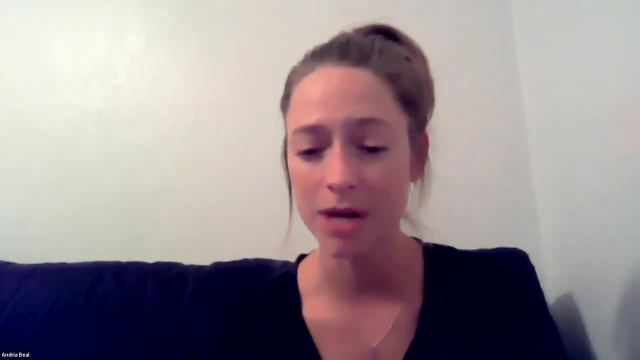 But yeah, there's a couple of studies out there, Um and actually I was putting together a lot of um collaborations. I was kind of talking with a lot of people trying to get samples to move forward with um doing age estimation for sharks. 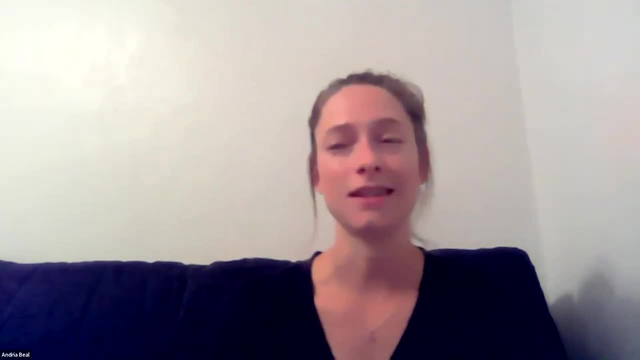 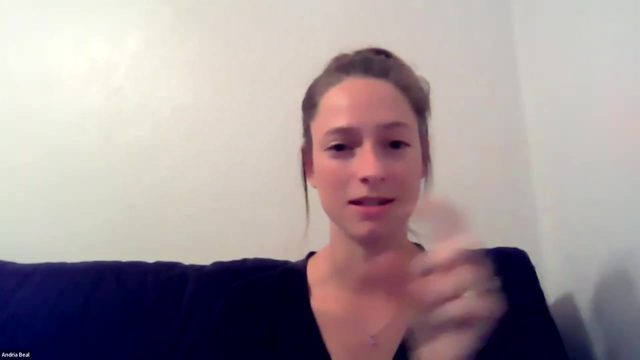 Mm-hmm, Which I, I will. I will someday visit this again and do aging stuff for sharks, I believe. Um, I'm still very passionate about the use of age estimation tools, uh, which uses that DNA methylation and we just um quantify it at certain areas of the genome. 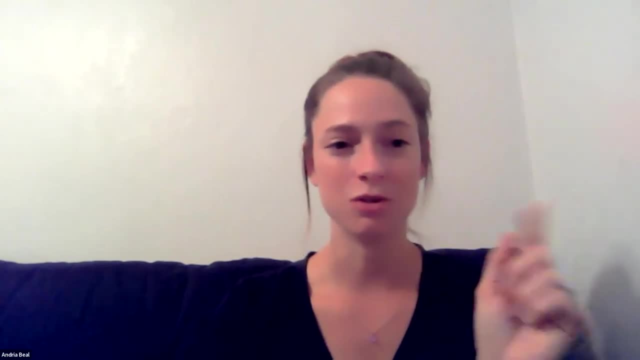 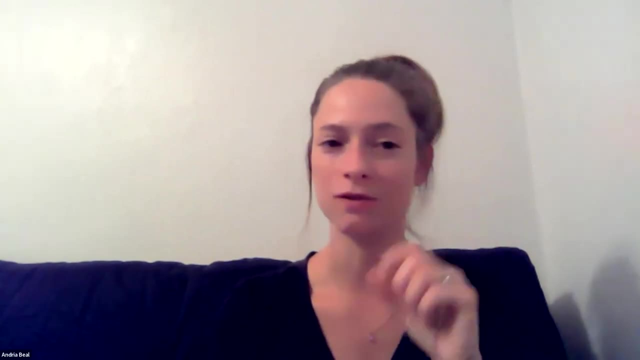 And so that's why we can't do a um age estimation tool for sharks just yet. Um, we're still. we need a little bit more reference genome data, because it's very specific Mm-hmm, And we we 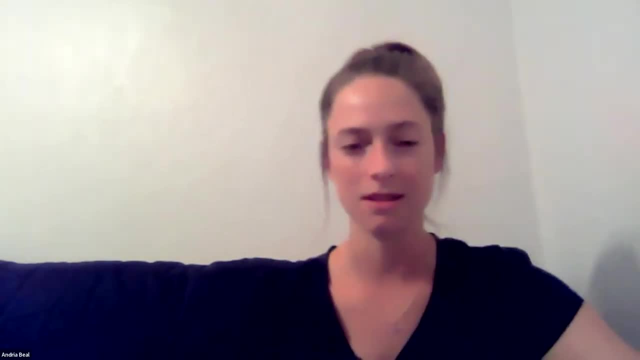 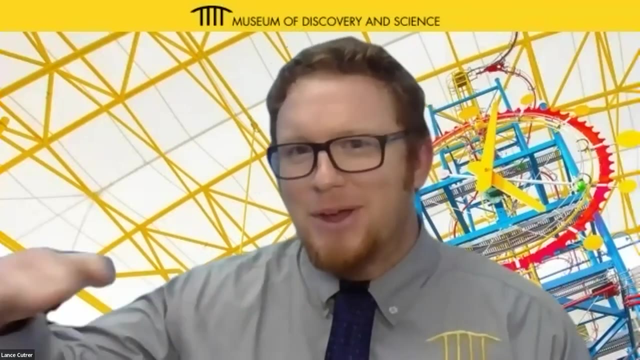 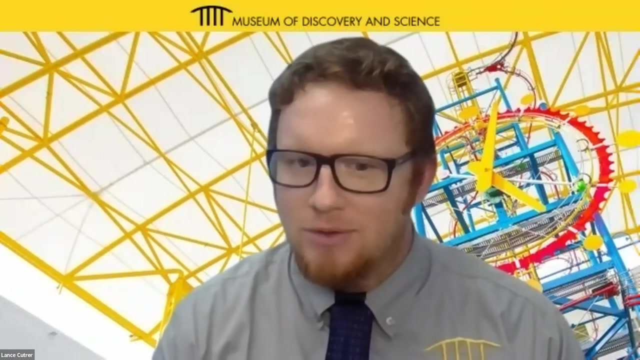 we need to measure that DNA methylation at very precise areas of the genome. Well, that's really interesting. So you so, with more research and that baseline study- right that you were referring to, getting that, that, uh, baseline data- you could look at a shark's genetic sequence and tell us how old it is. 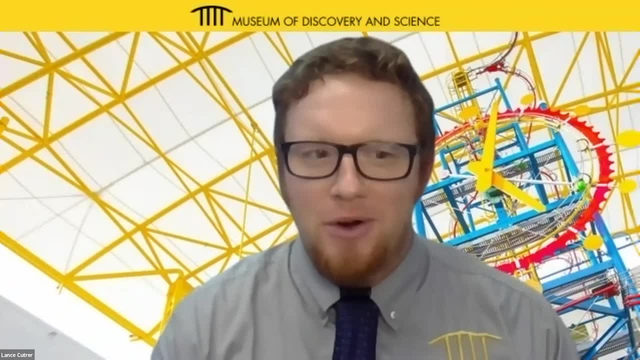 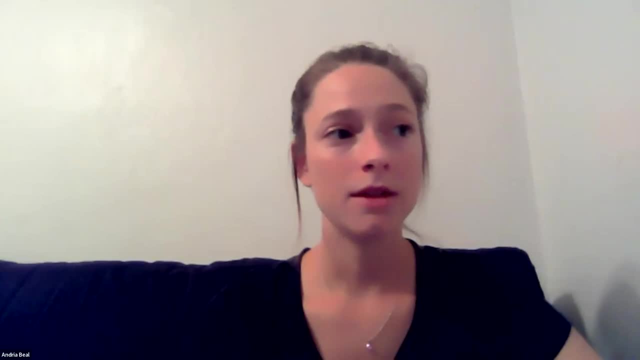 That sounds pretty amazing. Yeah, What, what's the? what's your, what's your range Like? is it like? what's your accuracy on that? Um, so with they actually so, with age tools like this, um, the most accurate age tools have been developed for humans, for forensics. 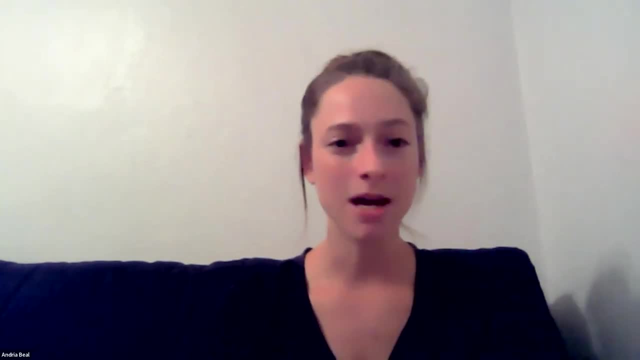 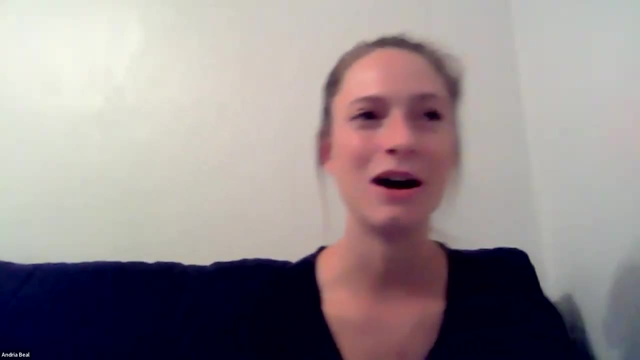 So that way, in that blood splatter, they can not only say oh, it's male or female, they can also say: hey, uh, they're also about 46 years old, Right, Or something like that. Um, and that accuracy is about at 97%. 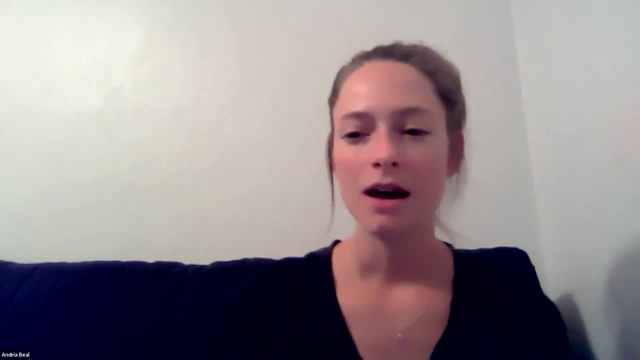 Wow, I think is the highest accuracy, 98%, maybe Um, And then we see with um, with um, dolphins, because I did an age tool for dolphins during my dissertation. Um, but since I did my age tool, that was one of my first projects in my dissertation um more studies with new technology came out in the age tool stuff for dolphins. And I think the lat. the latest accuracy for dolphins was at about 95 or 97% somewhere in there. They got Way up there. Um, the problem with really saying that accuracy is that we do notice that the age tests that they create tend to be population specific. 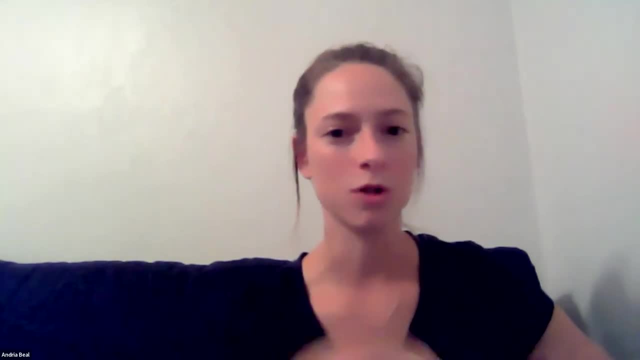 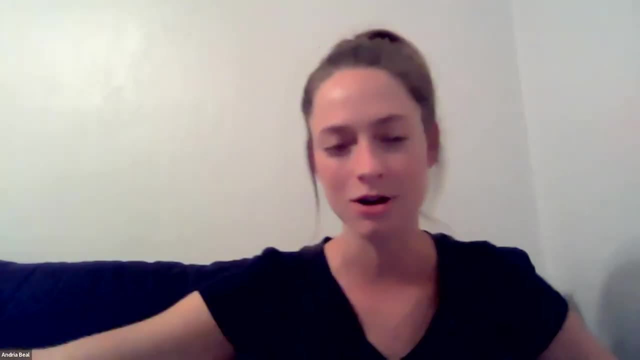 So we're still working on a better tool. That's more general. You see, um, you see that 95% accuracy with this one population, but then when you take it across the world and do it, um, you seem to lose some of that accuracy. 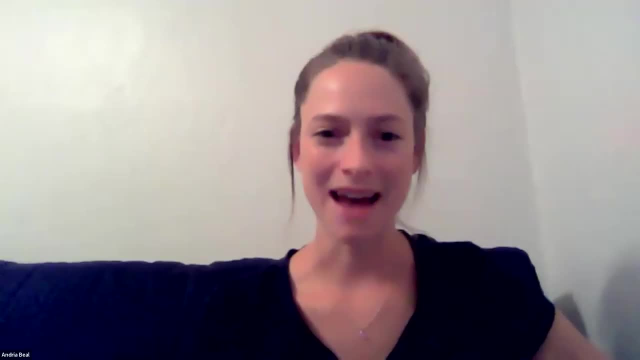 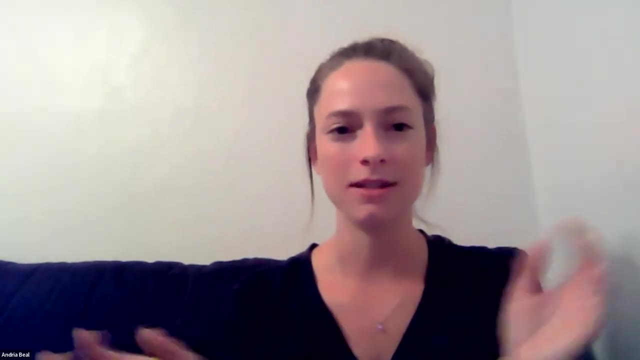 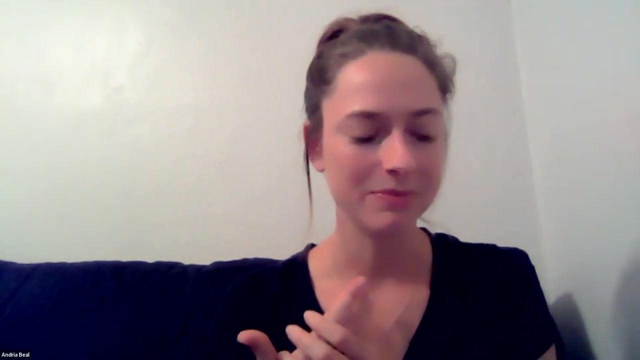 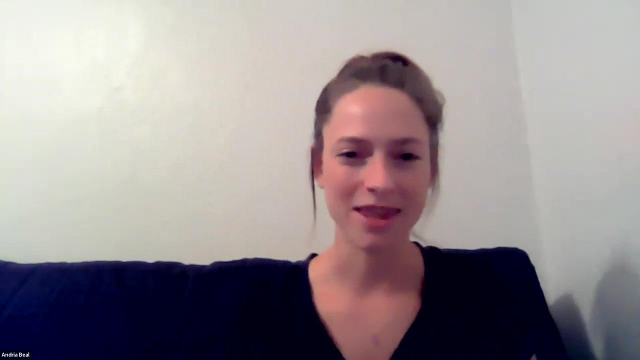 Right, Because the environment there is different, Right? Yep, exactly, So we're trying to isolate for parts of the genome that are very um correlated to that age and less of the environmental influence around that Um. but with aging, um, you know, we know that age is highly influenced by the environment. so it's hard to, it's hard to avoid that. 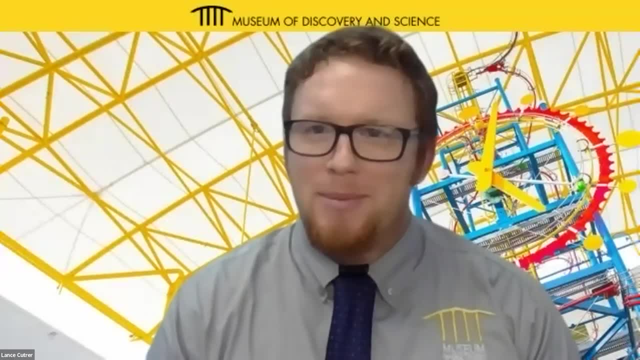 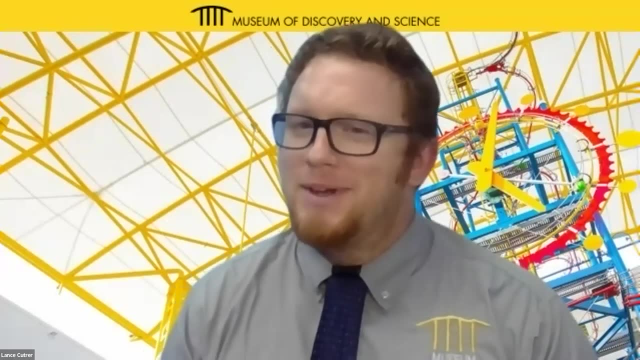 That's really, that's really cool. The power of genetics is. it's really amazing, It's, it's unending, like all the things you can figure out Just by looking at a DNA sequence and everything that's attached to it. 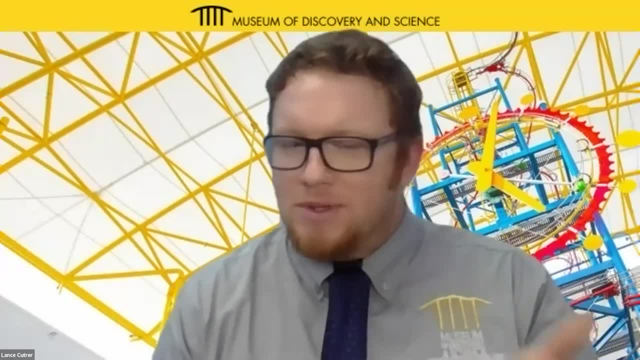 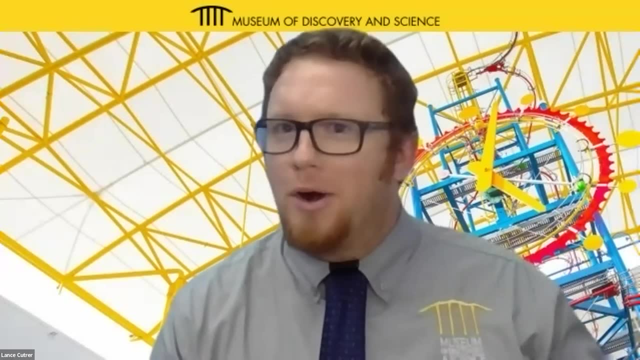 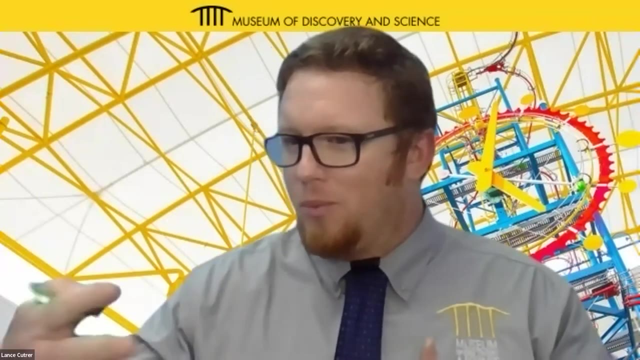 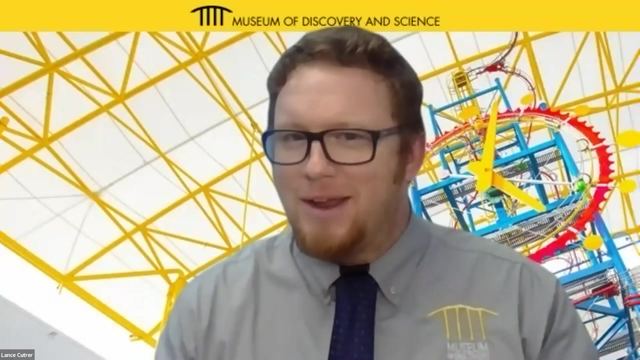 Um, I, I know just from personal interest that there you know, there's all this leading research with trace genetics and sampling water and looking at the DNA fragments in a water sample to say, oh, a, a shark was, or this species of shark was present in the water, just because we, this little small fragment of DNA was in the water. 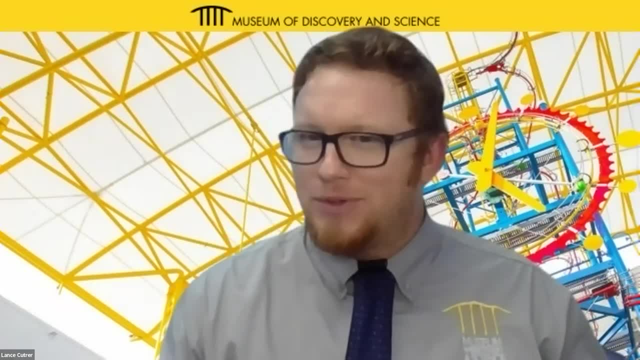 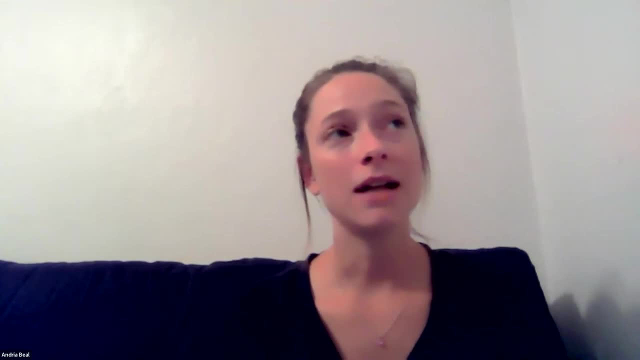 Right, Right, Yeah, No, And that's true. Um, I don't know of any studies trying to look at, So with that I mean it's little fragments of this or that. Um, I don't think that's enough to really help with the baseline for the DNA methylation. 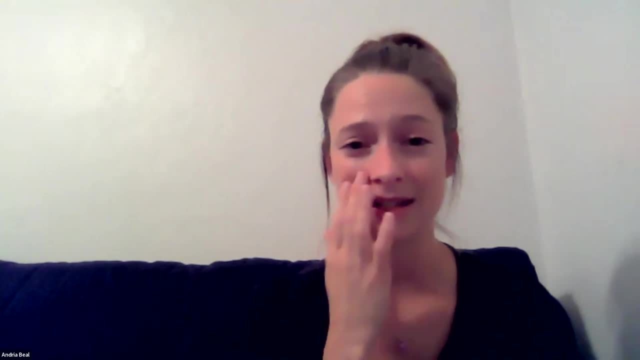 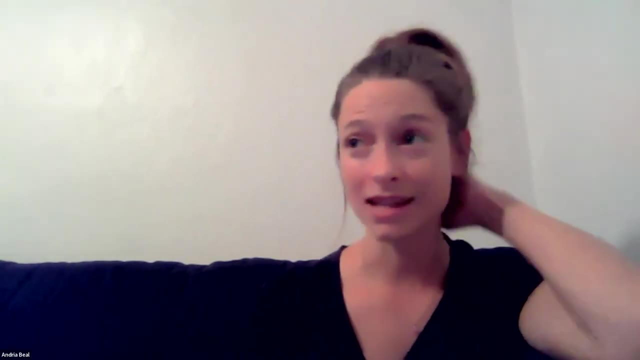 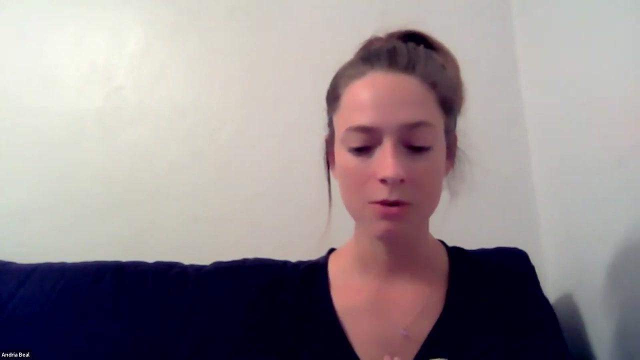 unfortunately, but it is really Right, Right, like that has just advanced our ability to know for conservation, you know what is possibly present. The last thing I heard about eDNA studies was they were trying to correlate what they found in the water with the number of individuals in the water. So not just: oh, we know this. 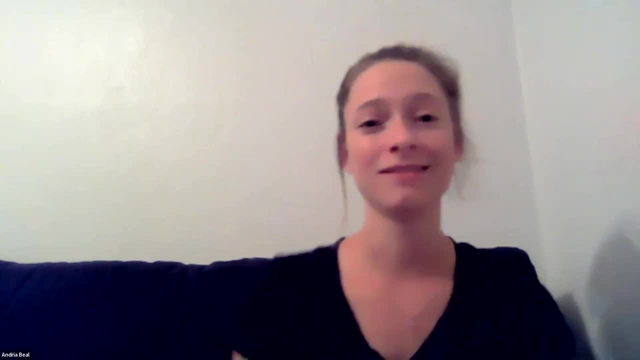 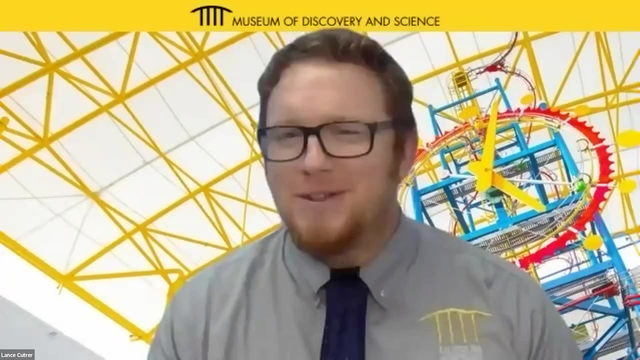 species is present, but there's probably 10 of them here. Oh, that's so amazing. That's really cool. Yeah, Well, that's super helpful to, for all kinds of reasons for sustainable fisheries, to know population sizes and catch limits. and, oh wow, Super powerful. Yeah, That's really amazing. 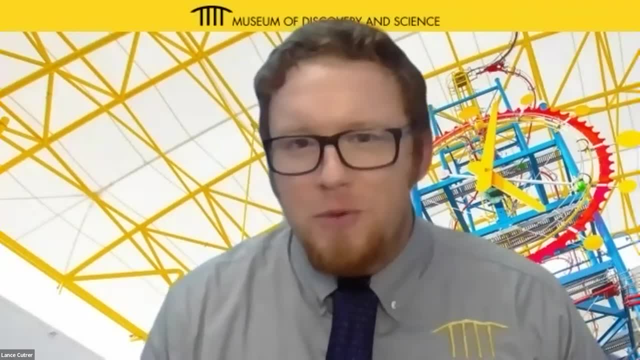 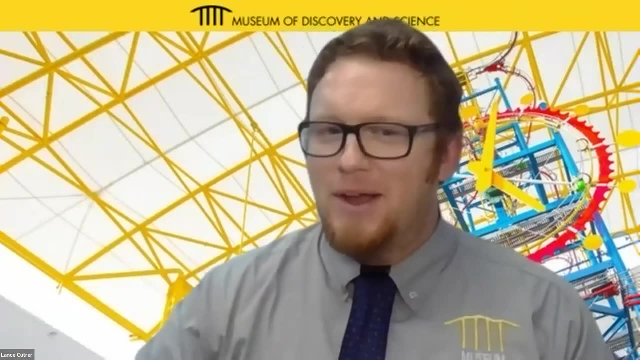 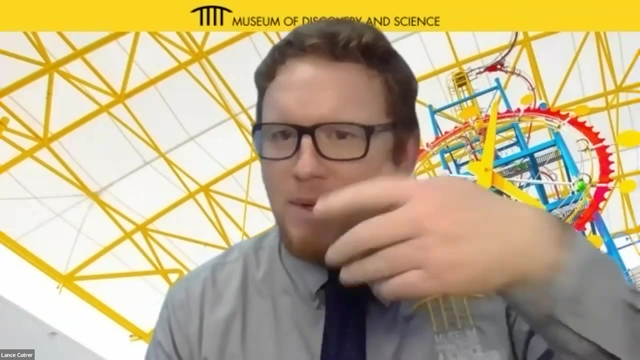 Yeah, Well, I do have a few more questions for you. I generally ask a lot of our distinguished speakers. some set questions that are a little more broad, And the first one being- you know, there could be some younger people in the audience that are really interested in. 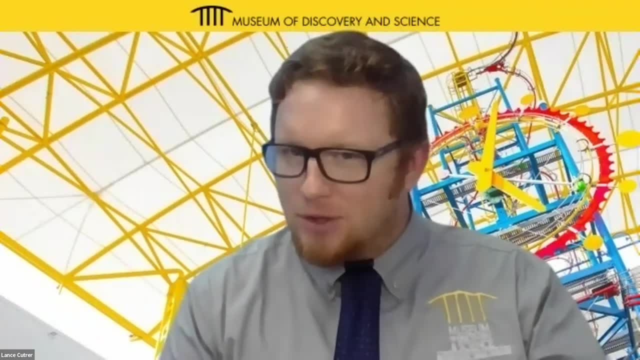 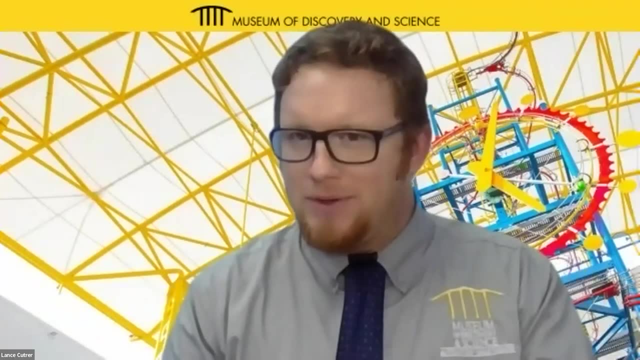 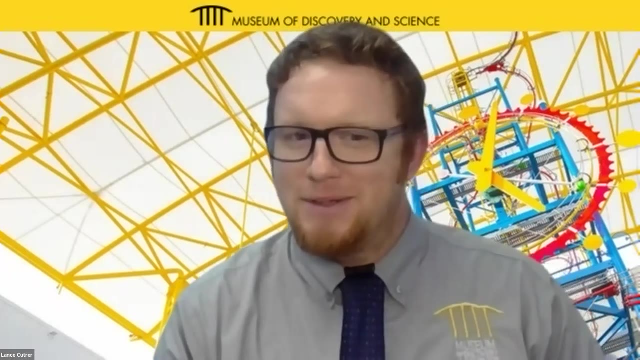 getting involved in this type of research, And so we're just wondering if you could kind of highlight your journey, Like: how did you get involved in this, How did you get involved in researching genetics of lemon sharks, you know, and looking for these things? And just in general. 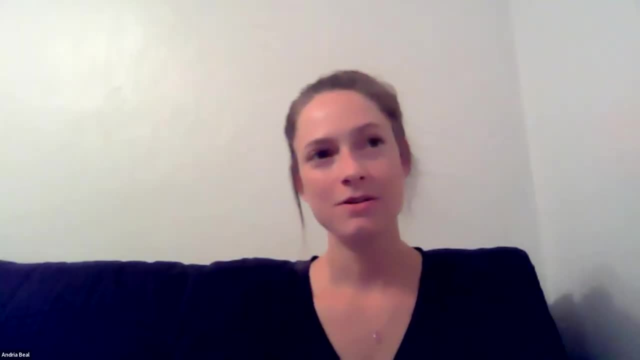 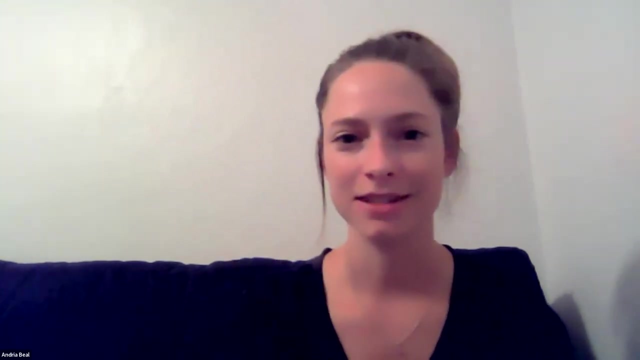 kind of tell us, tell us your story. Yeah, So I did my so. as an undergrad I started studying DNA in general and I was actually looking at population genetics in in cotton rats, So nothing marine at all- And then I went on to do my master's where 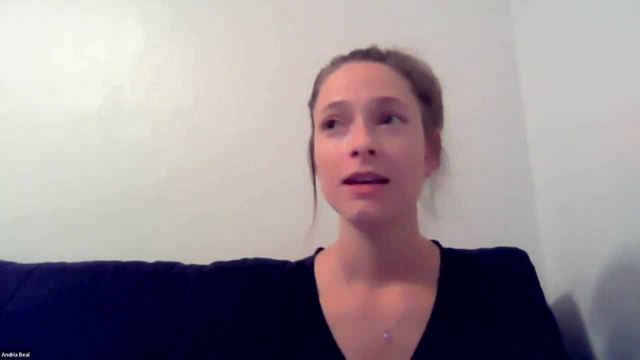 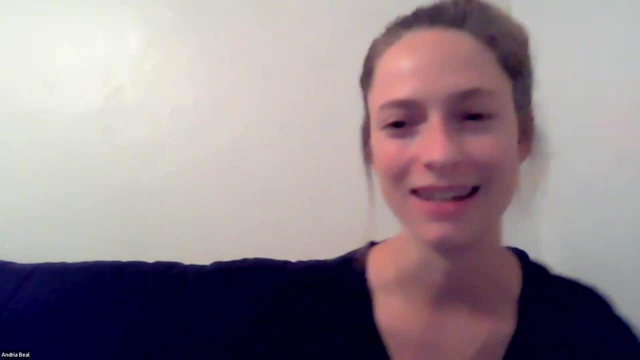 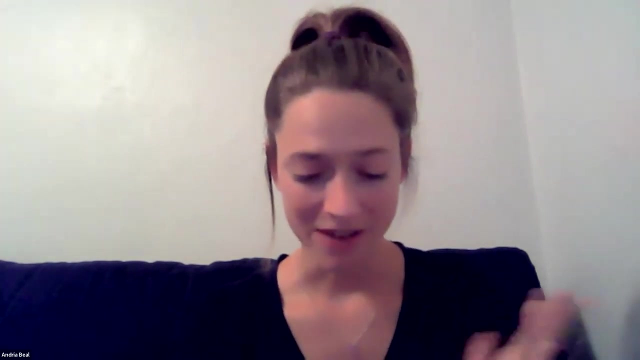 I started studying RNA And I did. I wanted to work with seahorses- so bad at that time but I ended up working with pipe fish, which are very closely related, and did the transcriptome for for um pipe fish And I compared male and females um brain transcriptomes And then from 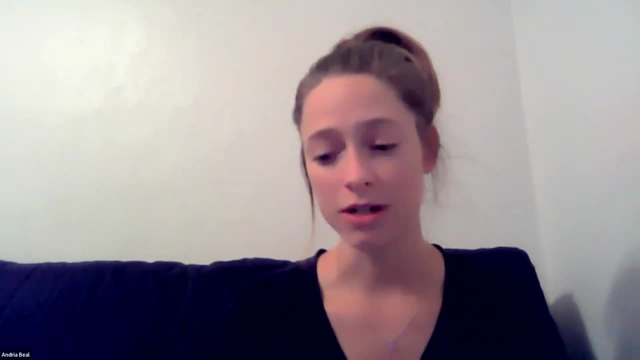 there I, I really wanted to work with sharks. I had always, you know, been partial to sharks and thought they were so cool. Um, I was living in Texas at the time, nowhere near the ocean, So, um, I started looking for a PhD where I could work with sharks, and I happened to. 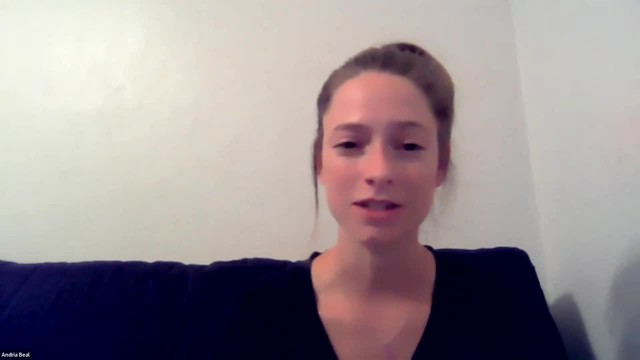 come across um the lab I ended up in, um Dr Aaron Lopez's lab, And he actually has a focus. his lab generally um studies a lot of coral, So not sharks, but um there was this ad for. 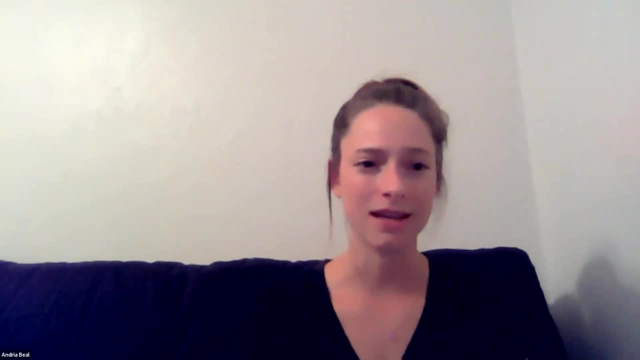 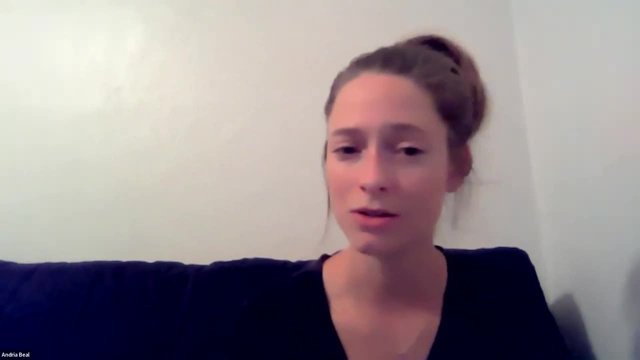 epigenetics, and that was actually what attracted me to his lab was epigenetics. I didn't know about epigenetics yet, So, um, I decided I wanted to check that out, And when I talked to him, it was perfect. He was just like: yeah, I'm open to. 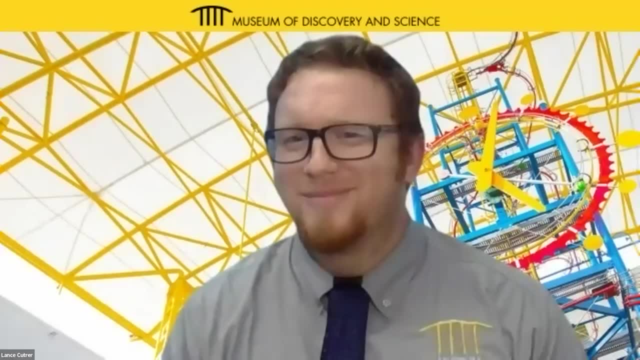 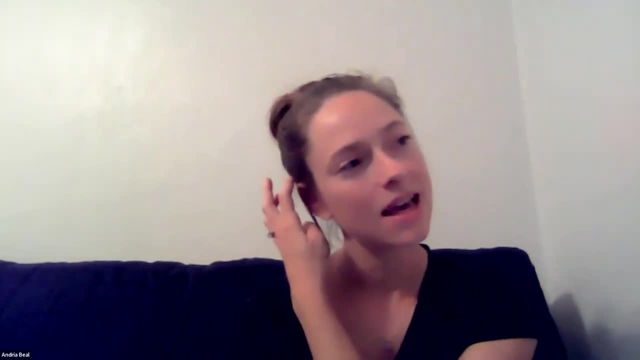 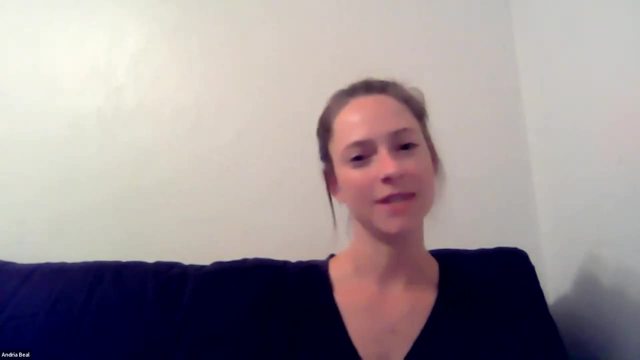 you can make your own study if you want. So I asked if I could try to do something with sharks or um. he had some work, I guess he had done with sharks in the past, And then also he was interested in um possibly doing something with uh marine mammals, uh from the other labs at. 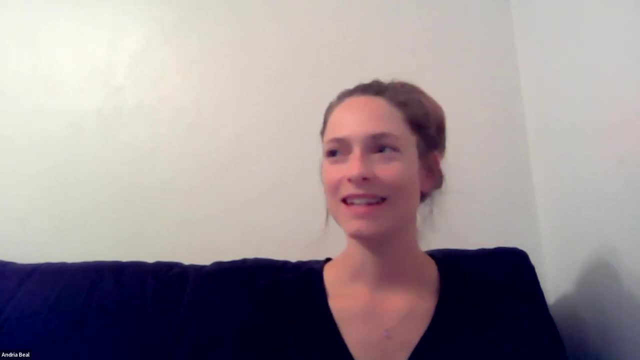 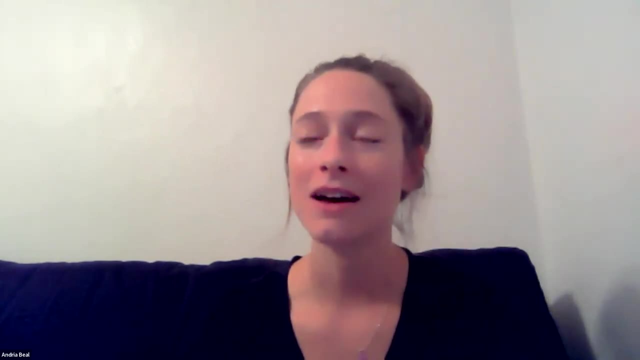 FIU. And so, um, yeah, he said I could do whatever I want. So I came, I said, all right, I'll be there, We'll give it a try, but yeah, definitely, Um, the best way to get into. 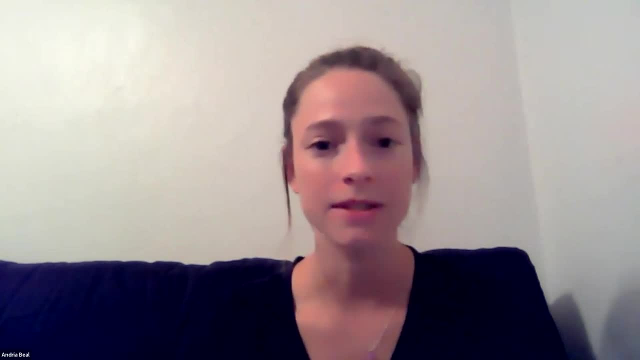 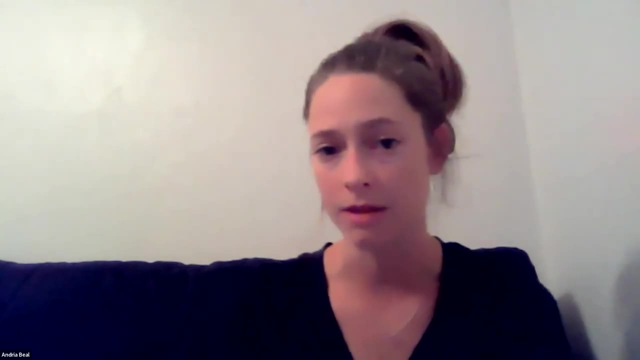 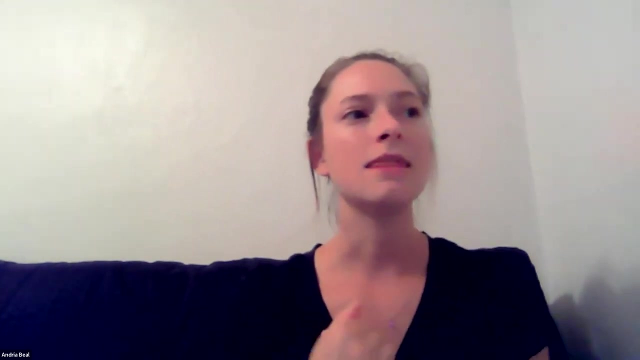 this is to start looking at different labs, Like say, if your starting point is so, I had two things. I had sharks that I really wanted to work with, So I was looking around in that direction. Um, and there's a lot of great shark biologists at FIU, which kind of led me over there. And then 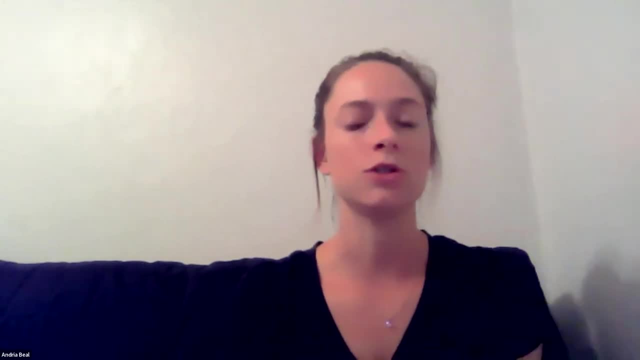 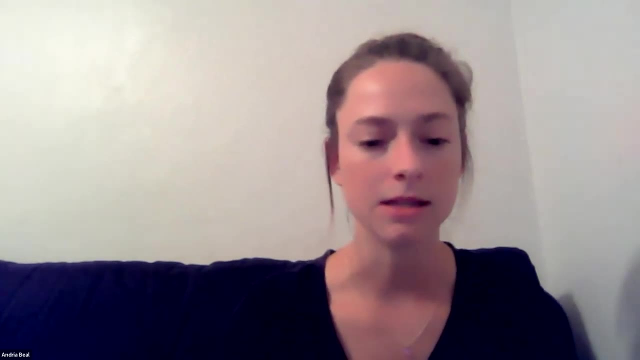 I came across epigenetics, another topic that I was just interested in, And so I, when I reached out, it just kind of came together: Um, and that's really how you get into something like this is to start looking for your interests and start talking. Um, that's how you're going to get. 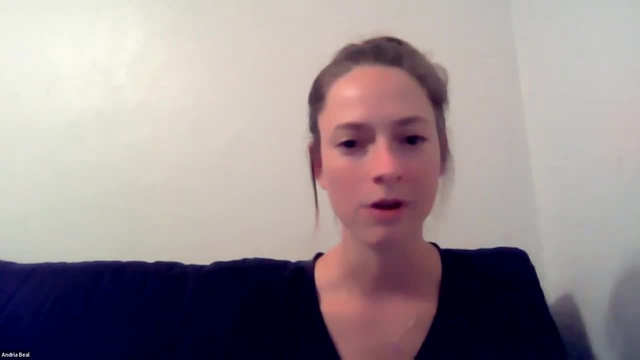 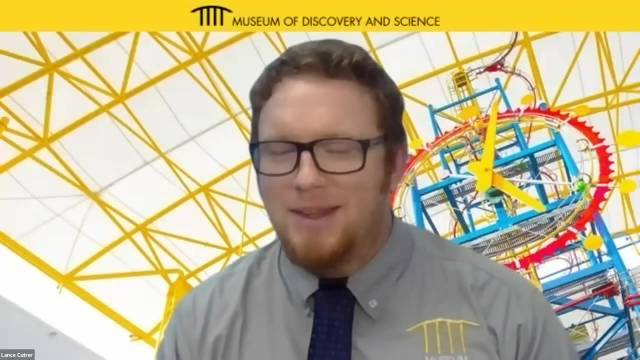 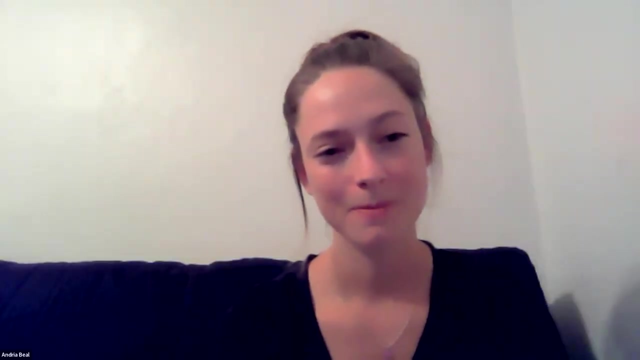 into a lab and be invited to do a upper level um degree like this. That's amazing. Yeah, So I, following your interest that that's been a a very common refrain from from all of our distinguished speakers. It's just like if you like it, go do it Right. 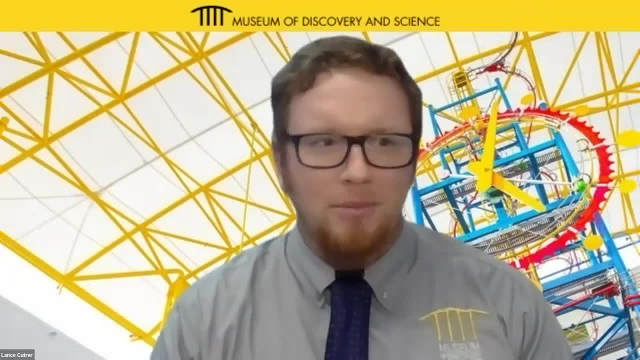 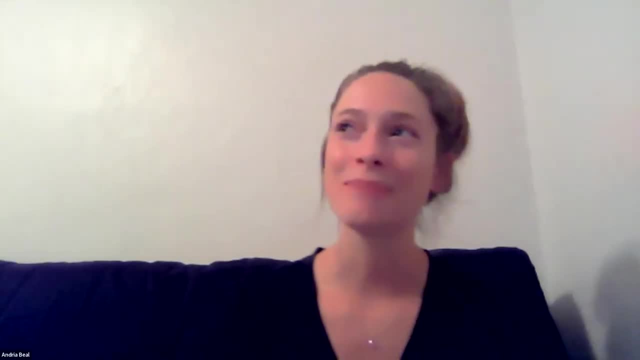 And whether or not you're young or not, like you should. that's a. that's a good life lesson In general. right, Try to follow something you want to do, because I'm telling you, no matter what you choose. 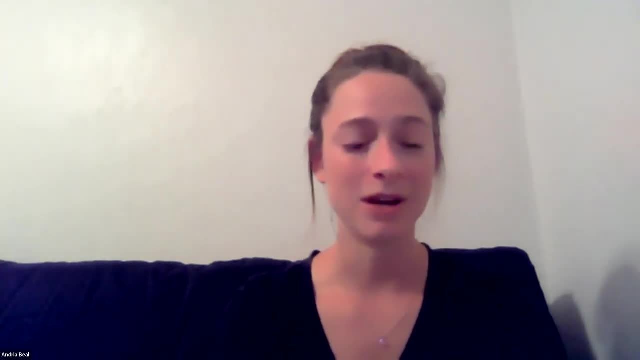 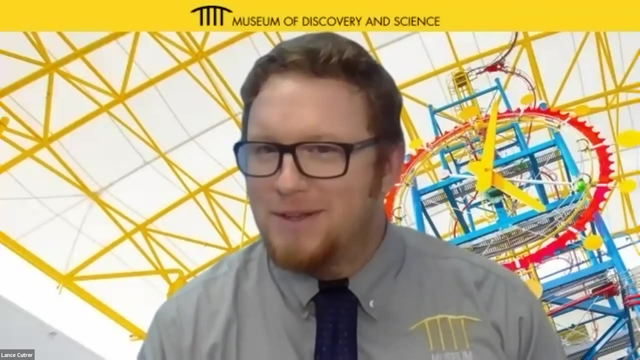 there's going to be challenges. So having a passion for whatever you've chosen to do, really it goes a long way And it was great that I guess it aligned perfectly for Save Our Seas to to fund your research too, Right, And that was. that was nice. 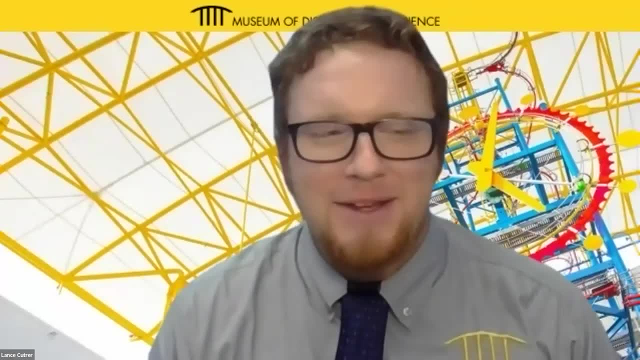 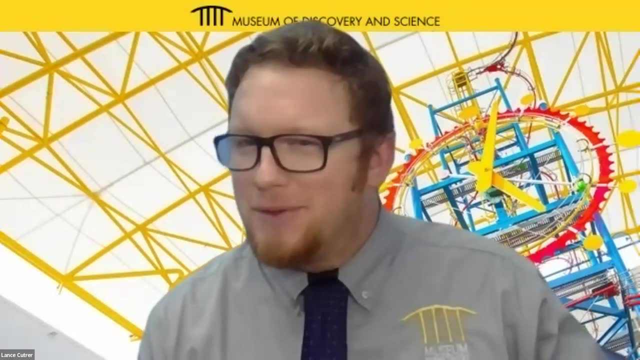 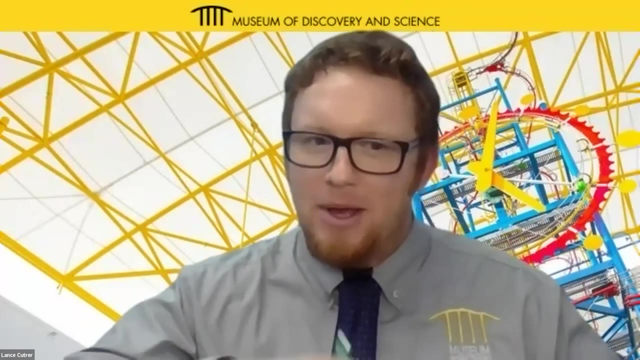 Um, well, speaking of funding and these kinds of things, so let's, let's imagine, uh, a scenario where you're, you're, you're given a blank check for this, for your project. How would you expand upon it? What would you do next? I think you kind of touched on that a little bit, but elaborate. 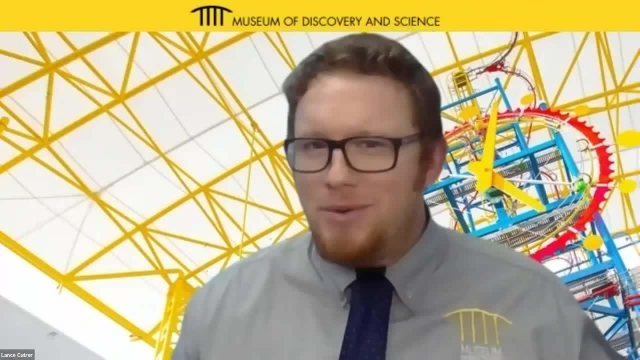 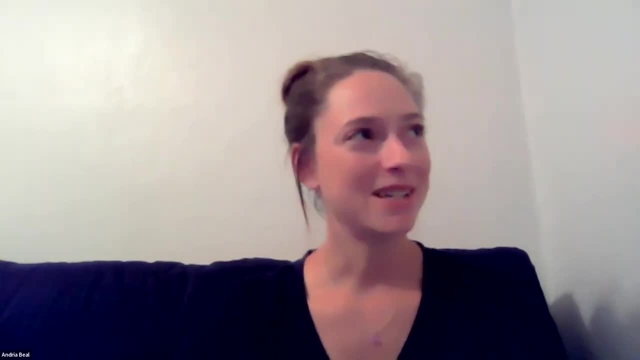 more on that, because you never know who's listening, Right? Um, what would you do next, Right? If? if you were given more funding to to continue your research? Absolutely. So during my dissertation I did apply a couple of times to do a reference. 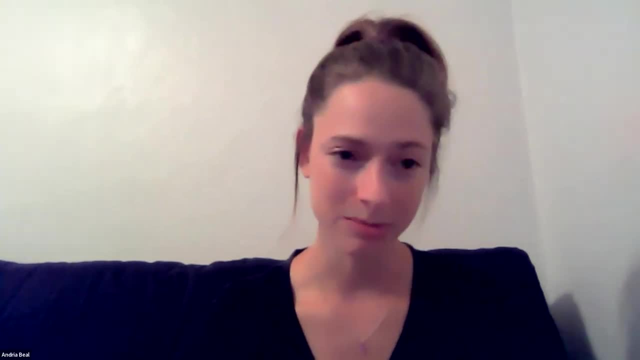 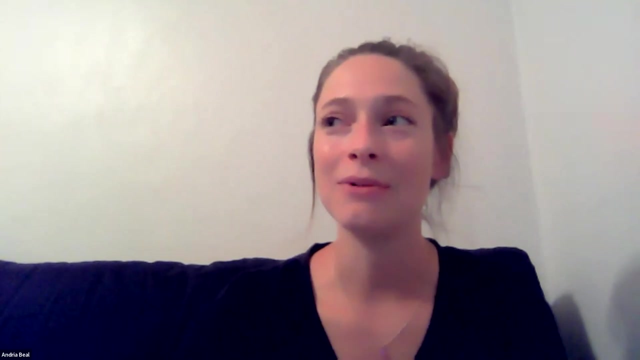 genome for lemon sharks, Um, cause they make a great model species For what we're doing. Um, especially with those archive samples that Bimini has, it's just the purple perfect, you know, experimental design right there with our dredging event and everything. Um, so I would definitely get that reference genome that we need. 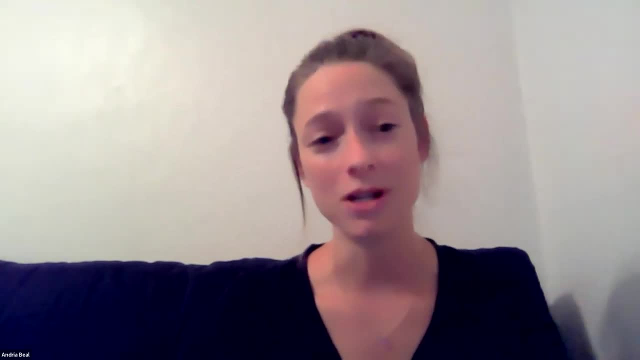 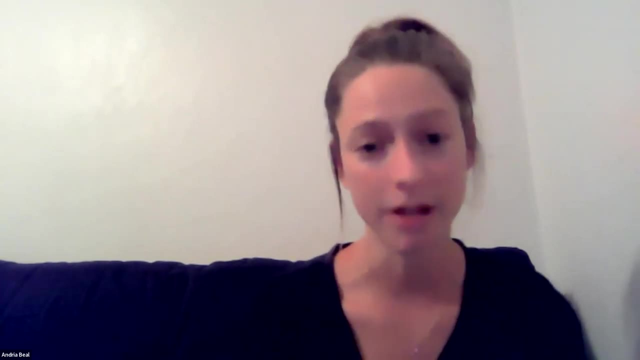 for lemon sharks. So that way we can go back and see you know what genes were affected by that dredging event and kind of try to get down to the bottom of whether or not trace metals played a role. Um cause that has. 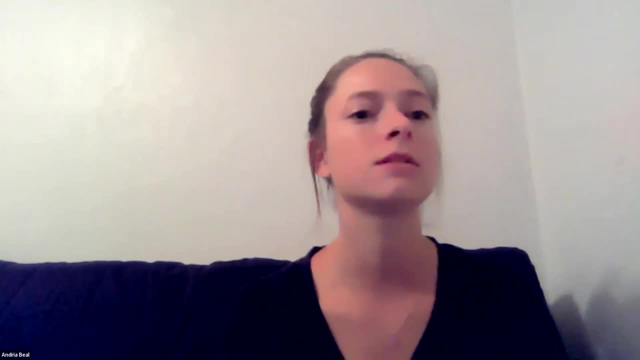 Implications for future dredging events. right, They do put up things to try and control um that um plume of of you know silt that comes up when they start dredging Um. but you know, it could be that trace metals really get reintroduced into the environment along with. 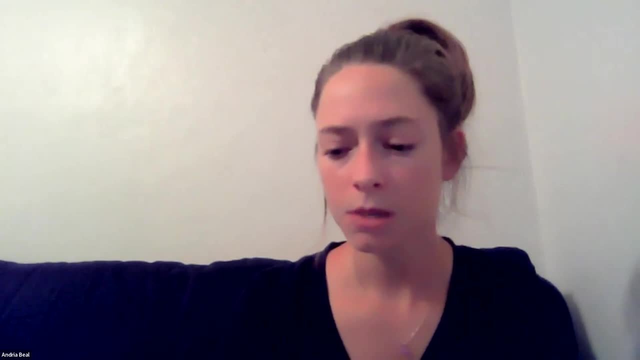 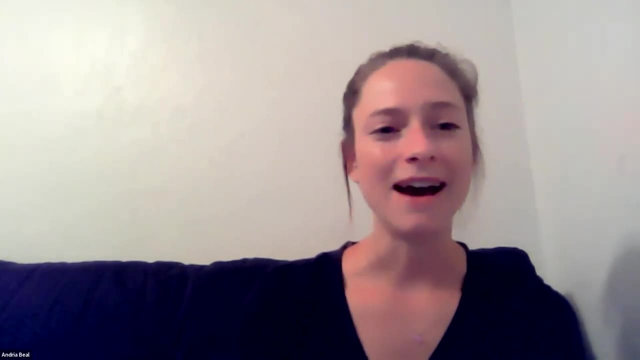 other pollutants. It could be other things too, Um, but yeah, trying to get to the bottom of that would be something I would do, And then I would definitely, you know, expand on that with that reference genome to get my shark age uh test done for sure, Like that's. 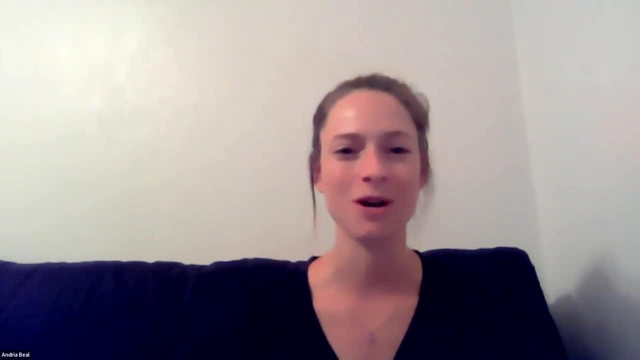 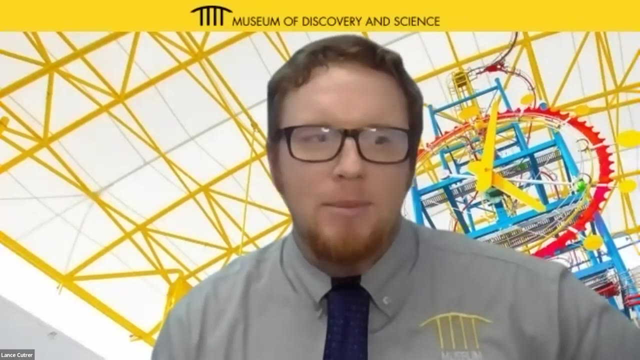 where my passion lies is using these age tools for conservation work. It's just, it's so powerful, It's game changing. So right, Yeah, It's, it's really interesting. I mean, you think about lemon sharks. lemon sharks are very common shark to see in coastal ecosystems Like we have here. 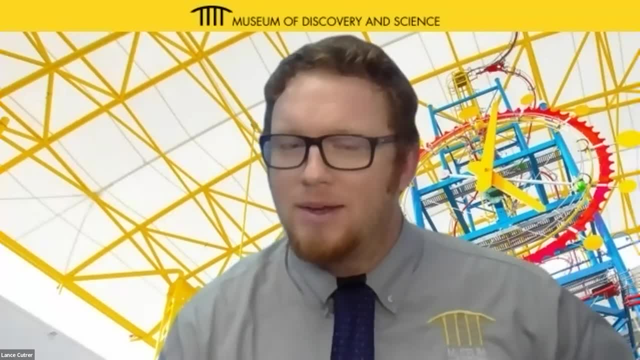 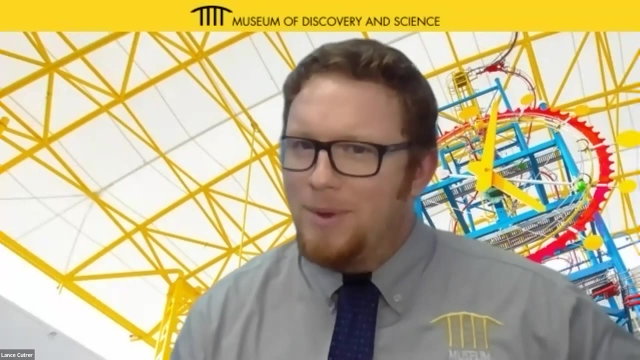 in Florida and in the Bahamas and beyond, right Um, they use these mangrove, these wonderful mangrove forests, as nursery grounds, And so, um, I can see how that species particularly would be really useful to have that data on um, cuz they're quite common. 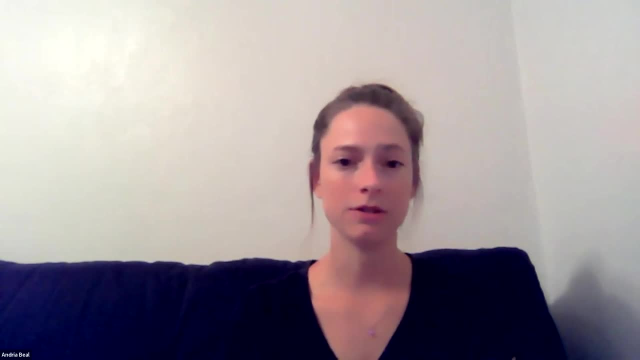 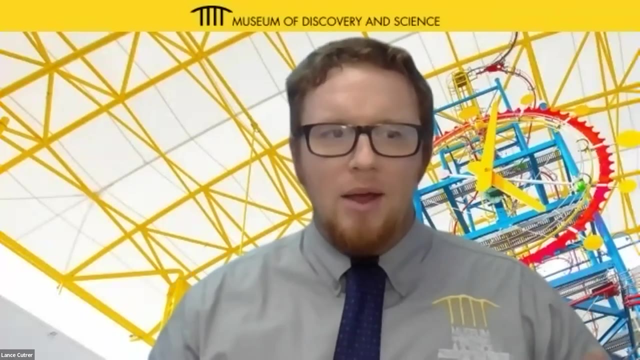 Um, yeah, they make a great model, just in general, you know, for shark species in general. you know, right, Cool, Um well, uh, one last question for you is: just how? how would someone that's watching? 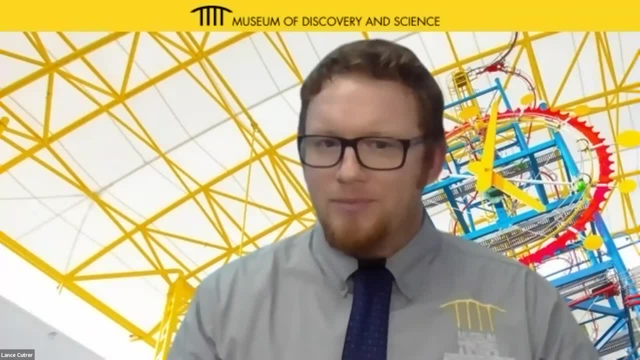 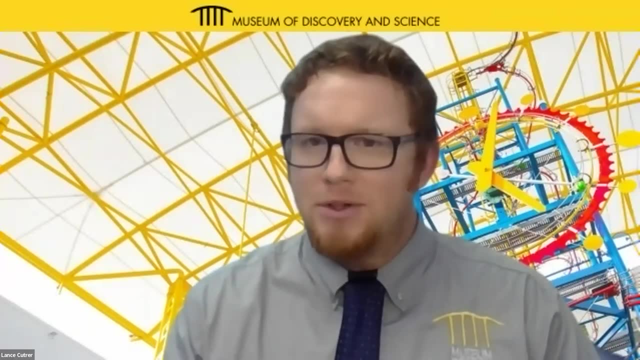 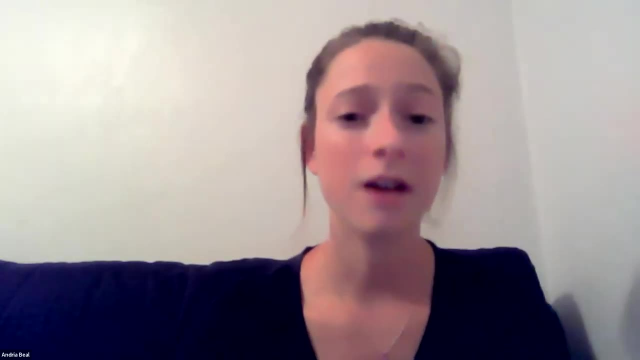 um, how, how could someone get involved in, in, in helping with this research or conservation with lemon sharks? Um, how could a general public take action and and help getting involved with this? Absolutely So there's a lot of foundations, um, including, you know, save our seas and you. 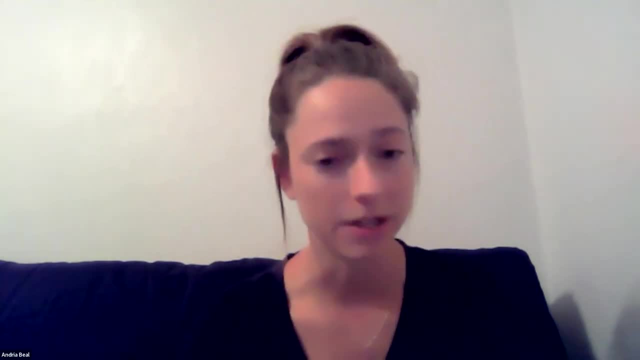 can always donate, like we need money for this kind of research. We need money for, you know, going out there and doing the frontline conservation work. to you know, stop um or intervene with some of the, the fishing that's. 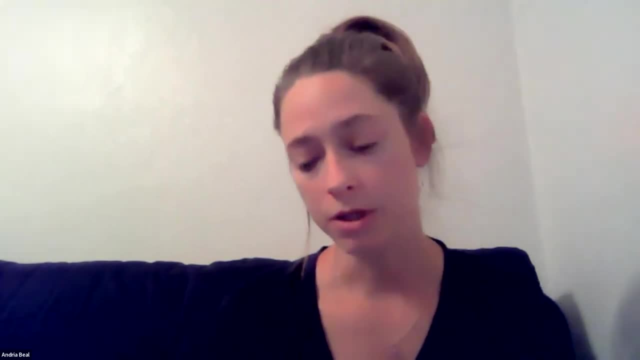 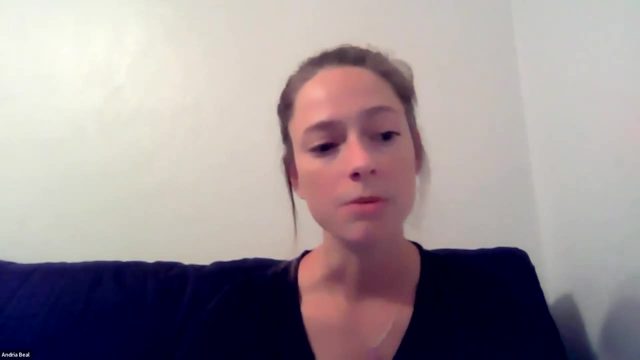 occurring that's really impacting populations. So you know money always helps, but then time- time is always. you know, great too. You can volunteer with these organizations, um, and come out and lend a hand. So definitely there's ways to get involved, Um, even the Bimini. 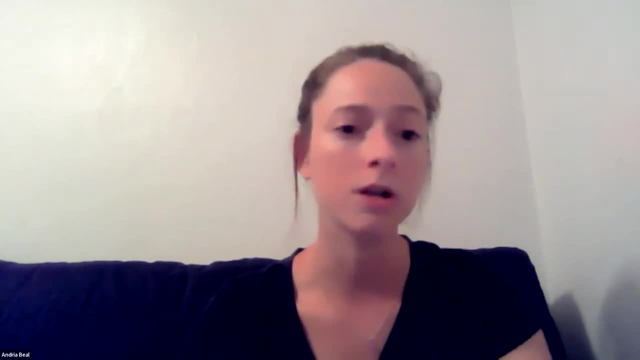 shark lab. um, you can go to them and they do tours. Um, you can definitely pay and have a tour and it helps them out a lot to to get that money and to do their research that they're doing. Do they volunteers as well? 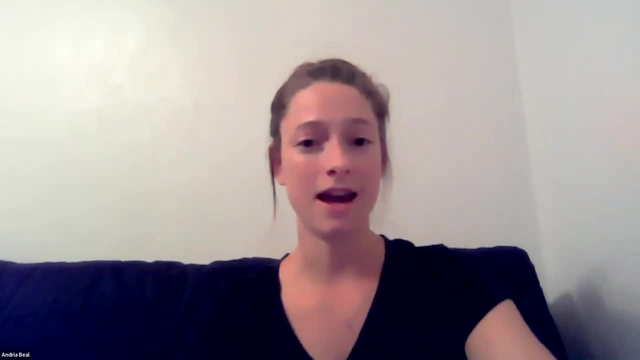 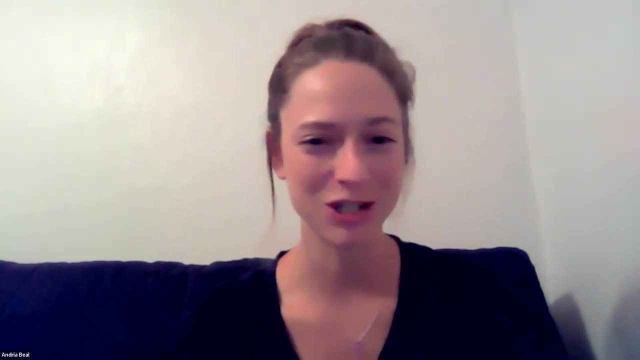 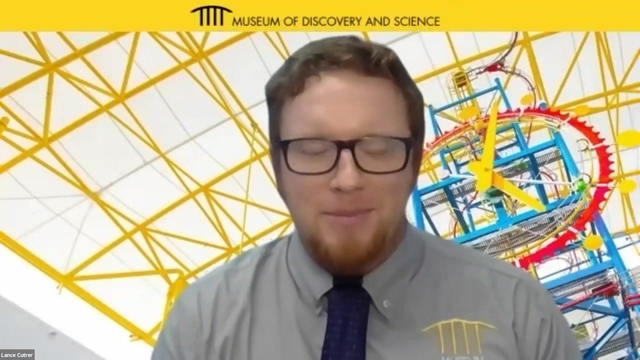 Oh, yeah, Yeah, They, they do volunteers, Yeah, They take volunteers. They have um citizen scientists stuff going on all the time. Yeah, It's really fun too. It's always fun to catch a shark, Right? Oh, that's really fun, Yeah, So just getting involved, uh, eating sustainable seafood. 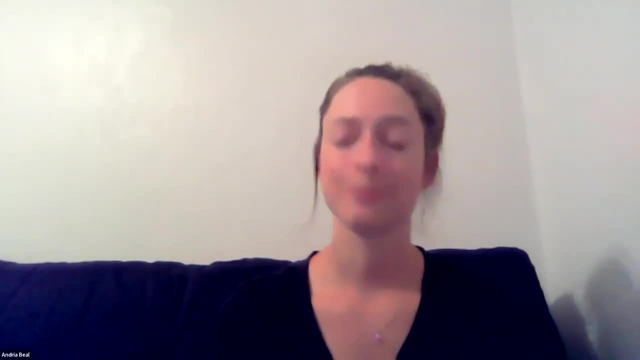 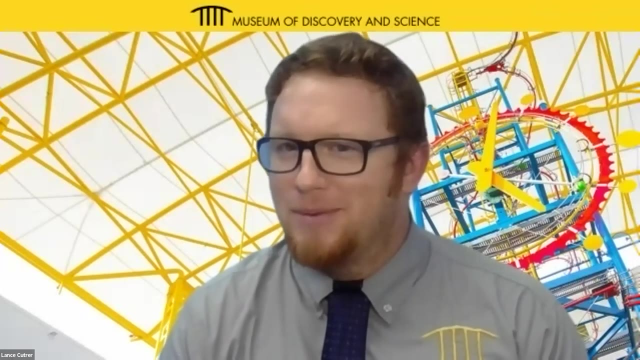 is a great one as well, right, Yeah, I mean it's really. it's really fun. I mean it's really fun. conservation: um, look at where your shark. we look at where your seafood is coming from, but to make sure it's sustainably sourced, and these kind of things as well i'm going to recommend. 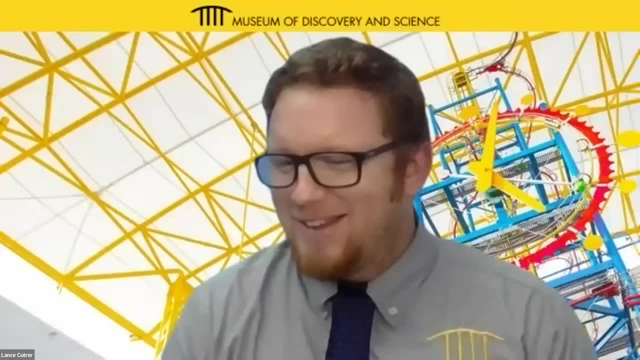 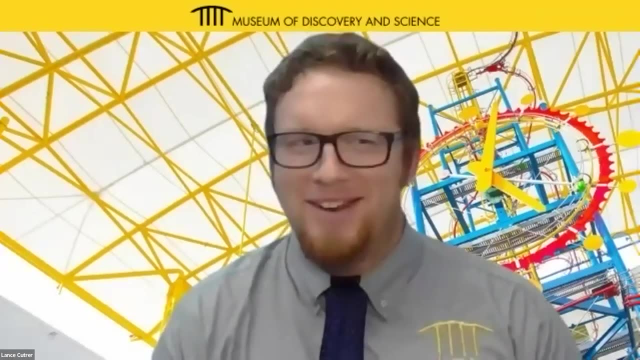 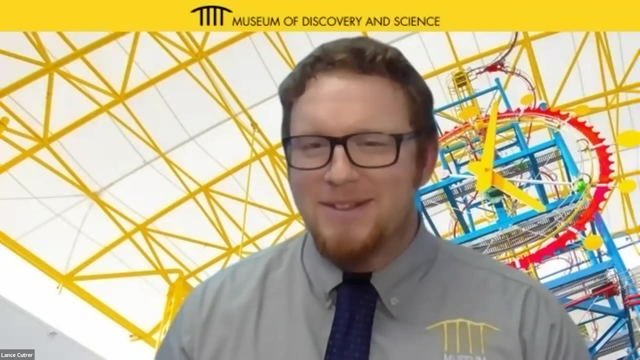 don't eat sharks. yes, to conserve sharks. let's not eat them, right? yeah, let's not eat them. yeah, they tend to have a lot of that first right, excellent. um well, thank you so much for for joining us this evening. um, going over your research, certainly appreciate it. um and all. 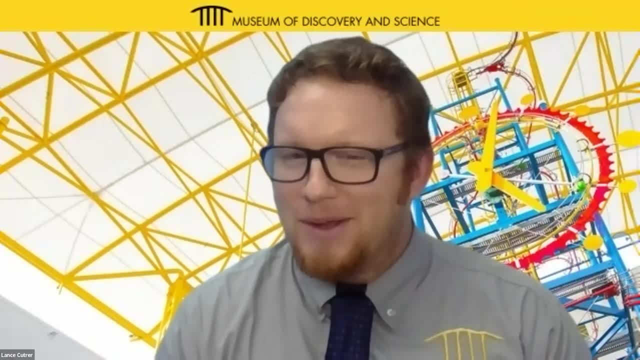 the work you're doing and good luck in your entrepreneurial um endeavors. right, that's that. maybe our guests can check out your website for um. tell us again what it was called: the the epipause, epipause, yes, to get some get some genetic information on on their pets, right, absolutely? 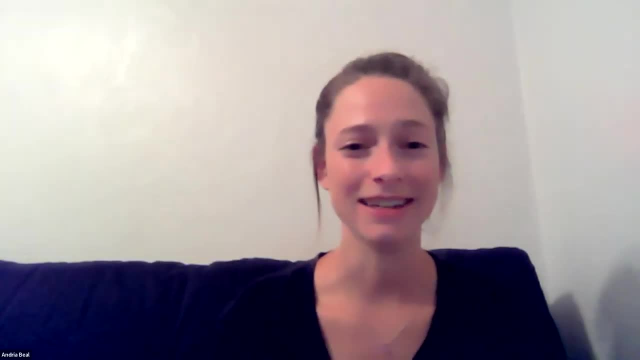 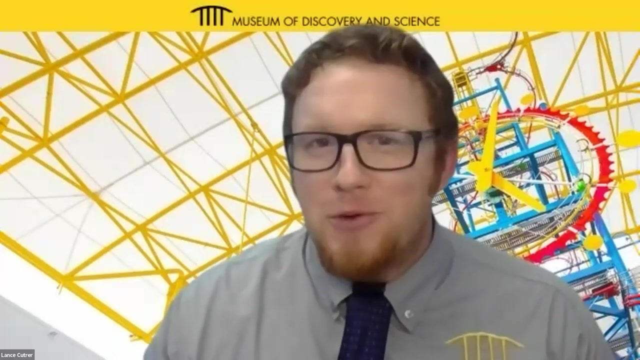 yep, and we're doing baseline studies right now. like, you can sign up your pet. it's completely free to participate in that research. um, definitely find something new about your pet. oh yeah, that's gonna be fun, right, excellent. well, thank you again very, very much, um, and thank you for all of all of you that have joined us this evening, just as a. 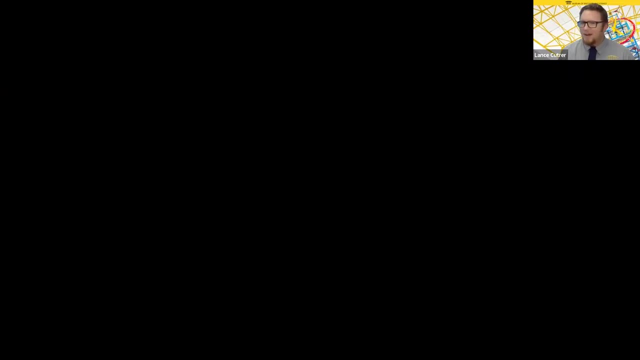 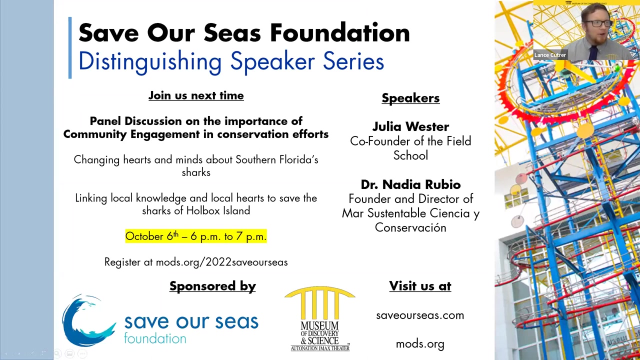 quick uh refresher for next time. so, uh, next month we are having our next speaker series, on October 6th, same time, same place, um, and this will be a panel discussion, so we'll have two researchers coming in, Julia Wester and Dr Nadia Rubio, to talk really about community engagement. 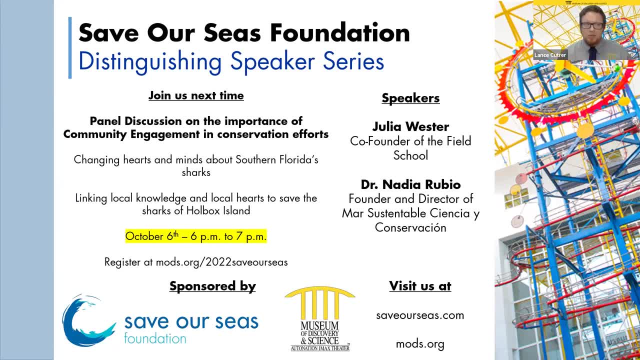 and how that goes forward and making positive change in conservation efforts. they are both involved in engaging community to learn from the community and to figure out how to best teach the community about conservation efforts. So we'll meet with them next time October 6th. 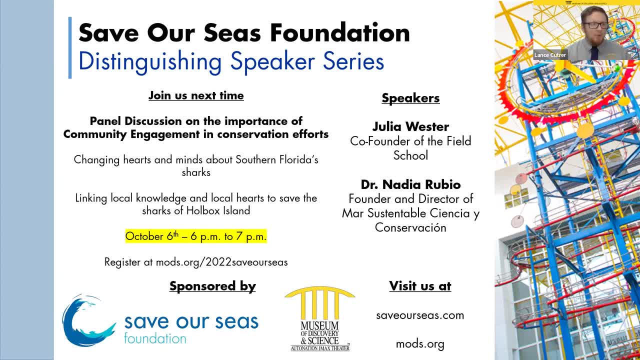 Thank you again to the Save Our Seas Foundation for sponsoring. Thank you again, Dr Beal, for joining us tonight, And thank you to everyone that joined us again. Hope everyone has a wondrous evening. Thanks for having me. Thank you so much. Bye-bye.